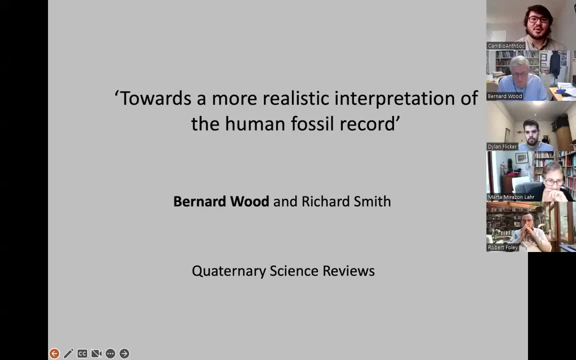 All right, so we'll go ahead and get started. So hello and welcome everybody. Thank you for registering for the Endless Forms seminar series hosted by the Cambridge University Biological Anthropology Society. We're an independent, student-led society dedicated to origins research. We offer a warm welcome to our guest speaker today, Professor Bernard Wood. 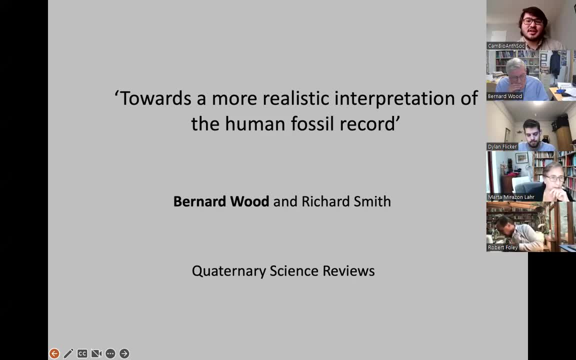 Dr Wood is the Director for the Center for the Advanced Study of Human Paleobiology at George Washington University, where he's the University Professor of Human Origins. Dr Wood is a medically trained paleoanthropologist who, while studying at the 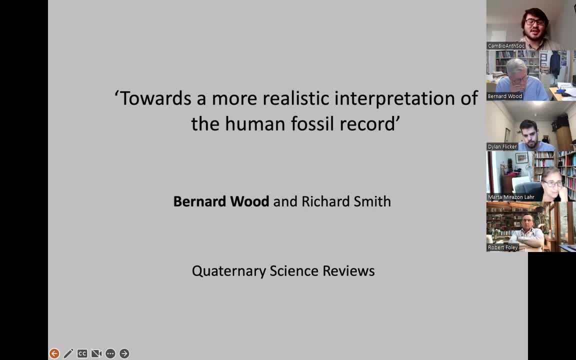 University of London was invited to Kubifora by Richard Leakey. Working with Michael Day, Philip Tobias, Alan Walker and other researchers, Dr Wood has contributed significantly to our understanding of hominin systematics and human origins. I'll now hand the time over to Dr Wood. 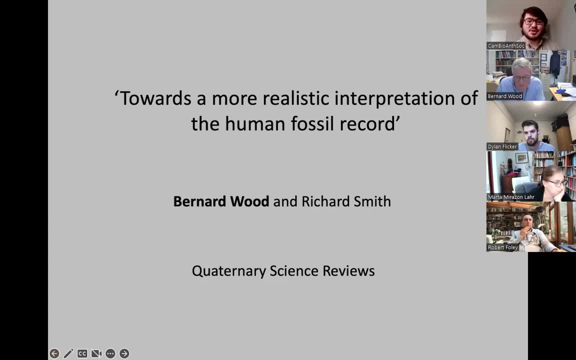 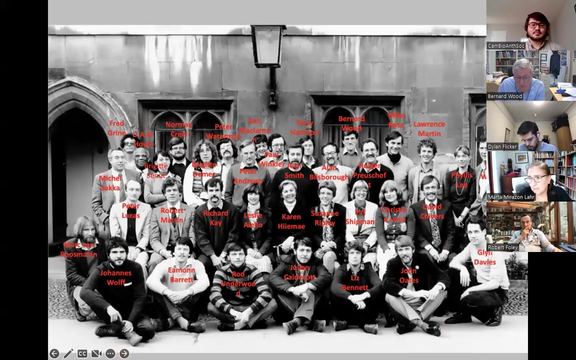 and we kindly ask that all questions and comments be saved for the Q&A session. Thank you for your invitation. This is the second of a pair of papers by myself and Richard Smith, and I will just introduce you to Richard Richard Smith, and here is a picture which was taken in 1982 at a meeting which resulted in this: 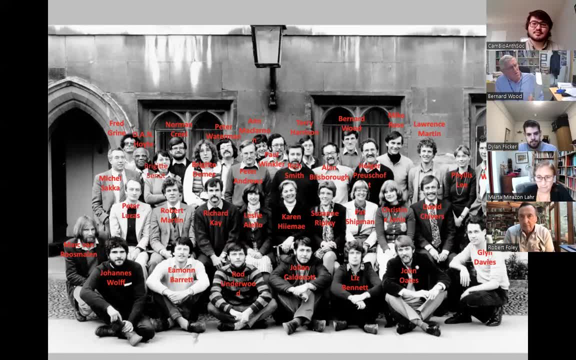 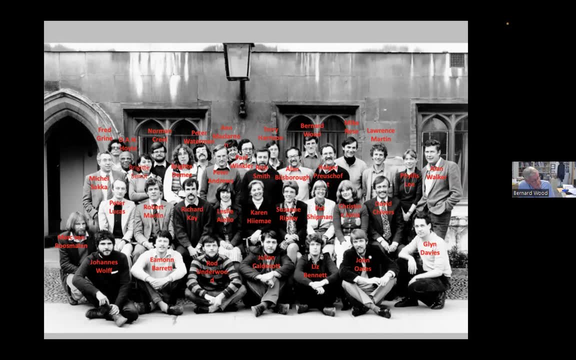 book Food Acquisition and Processing in Primates, which was edited by Alan Billsborough and David Chivers and myself on the top row about just over halfway. well, halfway you will see terry harrison and there's me next to terry harrison, but that's not the point. um, richard smith is the guy here and he. 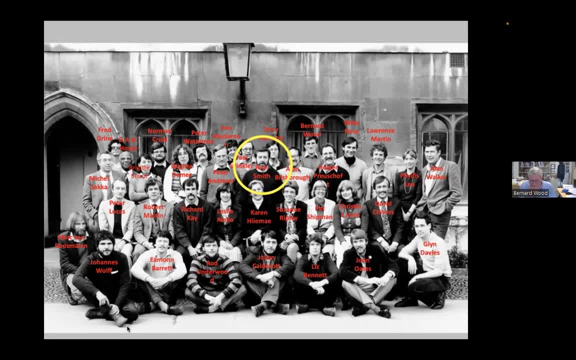 was at the meeting and um, he and i have been colleagues for a long time. um well, we haven't been colleagues in a sense, but we have been sort of co um um, we have been intellectual colleagues. we have never worked at the same institution and um. this is the second of two papers. the first one was about sort of epistemology. 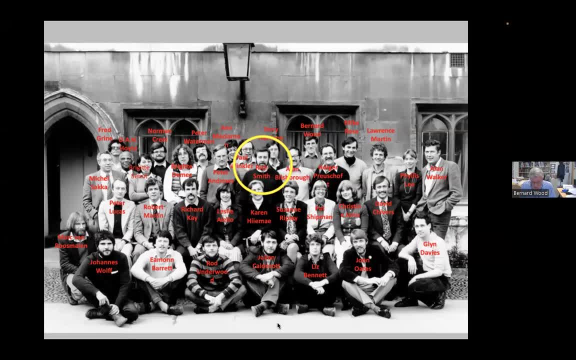 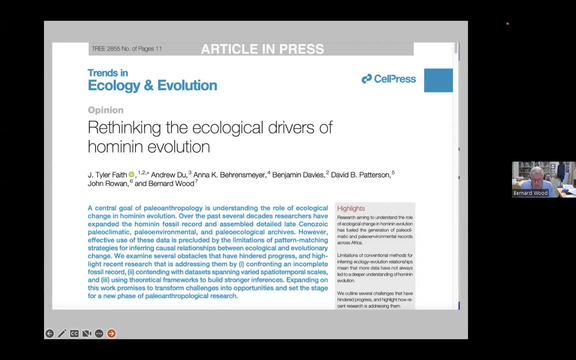 about what sort of questions you can actually answer in relation to human evolution, and this one is a. um is expands on a contribution i made to a review, um, the. the lead author was tyler faith and the other authors are um colleagues, um of mine or ex-graduate students. 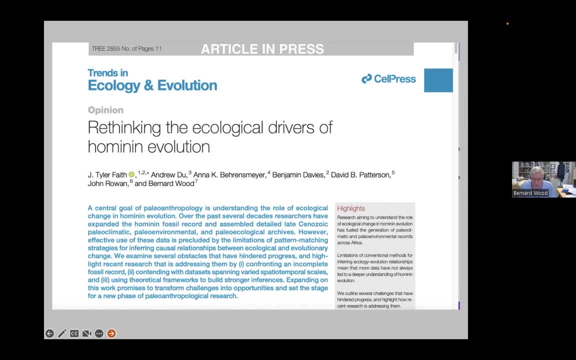 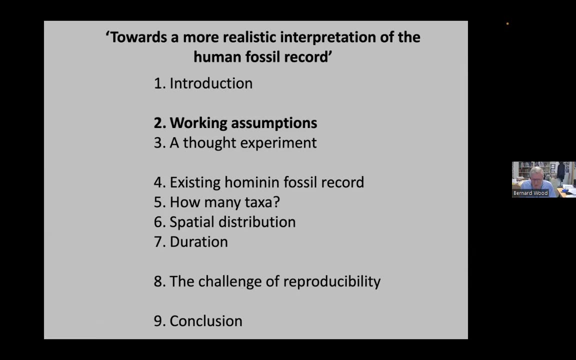 in our program, um, and graduate students of ex-graduate students, um, and the point of this paper is for us to take a realistic look at what the human fossil record actually can tell us, or what it consists of, and therefore, um, if we understand what it consists of or what it doesn't tell us, uh, then we might, um, then we. 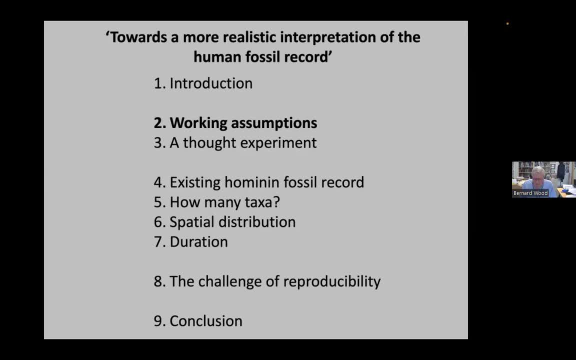 might be able to use it a little more, little more, um, sensibly and profitably. and the first thing, if you read the paper- and i don't blame you if you didn't- the first thing was that, um, what we did was to make some sort of assumptions, um, and the working assumptions are that that 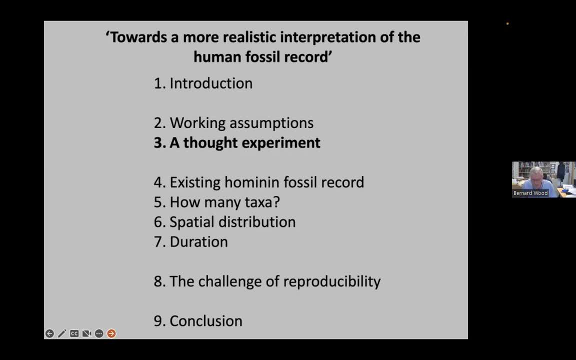 modern humans are most closely related to chimpanzees and bonobos and that their common ancestor existed in africa around six or seven million years ago. so that's the working assumption. and the working assumption is that, unless hominins for some reason left africa, uh, the 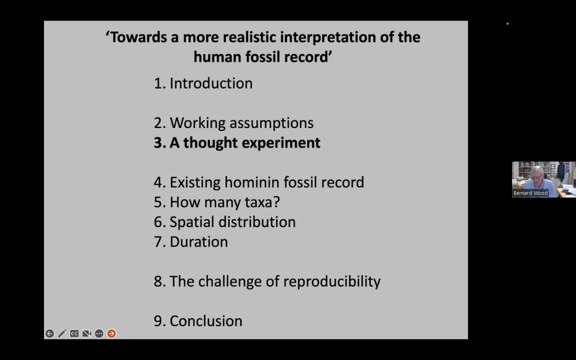 should be a fossil record of the hominin clade somewhere in africa for seven million years after that most recent common ancestor. so that, so those are, those are the working assumptions. the, the, the thought experiment is the following: um, and the thought experiment is really, is really an attempt. 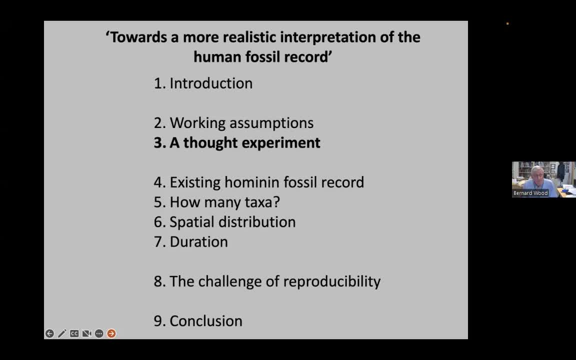 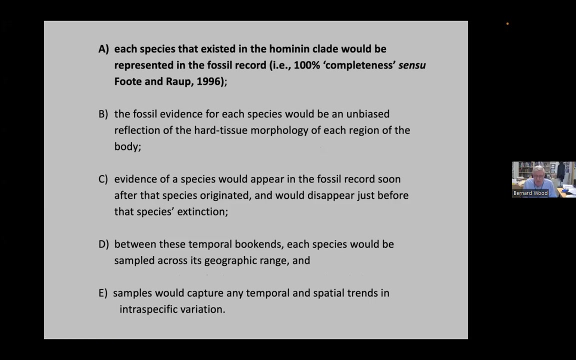 to come up with a, a, um, come up with a scenario which we can compare the, the existing fossil record to, and the and the scenario um. the scenario is the following: that each species well, and the other part of the. the working assumption is that, therefore, if there is a most recent common ancestor, 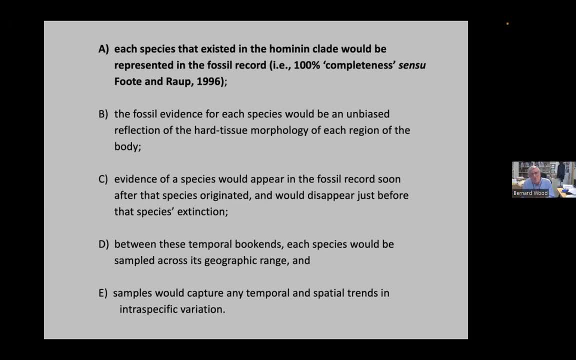 of modern humans and chimpanzees and bonobos. the assumption is that that common ancestor lives in africa and the assumption is that, at the minimum, in order to get from that common ancestor to modern humans, you must have a sequence of ancestors and descendants that connects you. 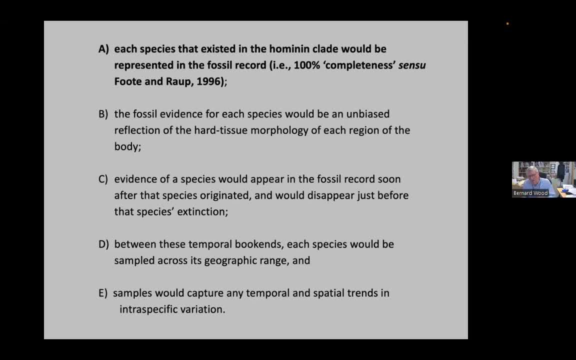 in other words, if you're seven million years ago, that sequence will take you to the present, and if you're at the present, that sequence will take you back to to the hypothetical common ancestor. So those are the working assumptions, The thought experiment, and so 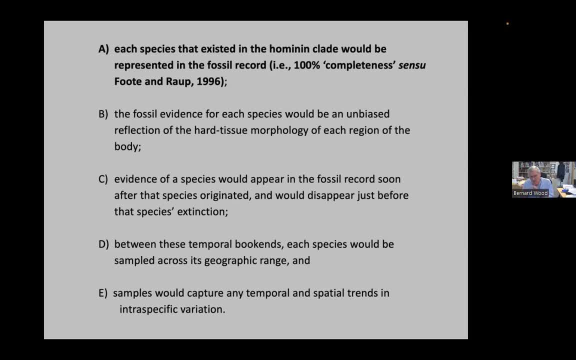 and the other working assumption is that at the minimum there has to be that ancestor descendant sequence. In theory, that doesn't have to be any other hominin in the fossil record. In other words, at the minimum you need just one chain to take you back. 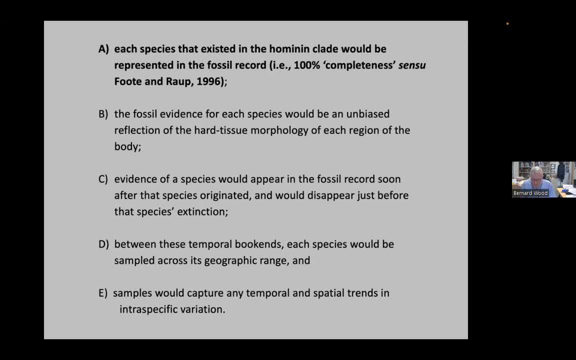 to the common ancestor. So what is the thought experiment? Well, the thought experiment is that each species that existed in the hominin clade would be represented in the fossil record. And what I'm telling you today is not rocket science, and it's been thought of a lot by other paleontologists. 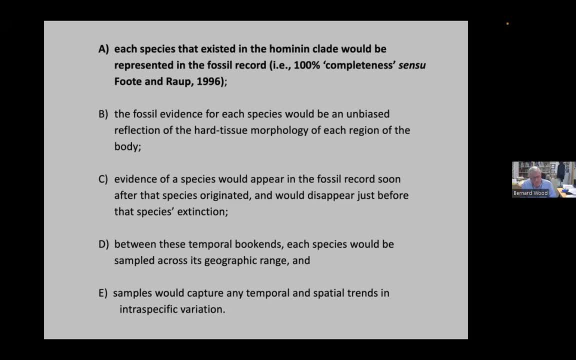 but not really, but by paleoanthropologists. Paleoanthropologists, and I include myself, are not the most introspective of people, And so, therefore, they tend not to look around them and see. well, paleoanthropology is a branch of paleontology. 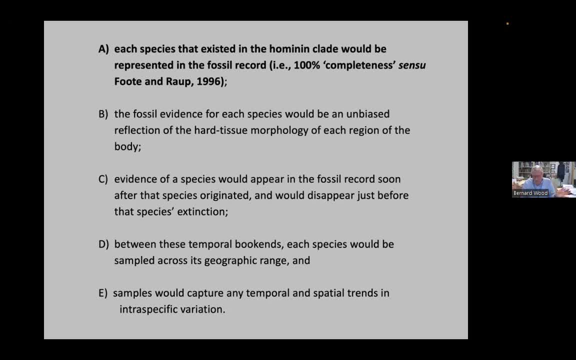 Let's see what other paleontologists are doing. Paleoanthropologists have a tendency to have tunnel vision, or at least partial vision, but partial tunnel vision, And I include myself in that, And this is an attempt to, in a sense, get away from that. 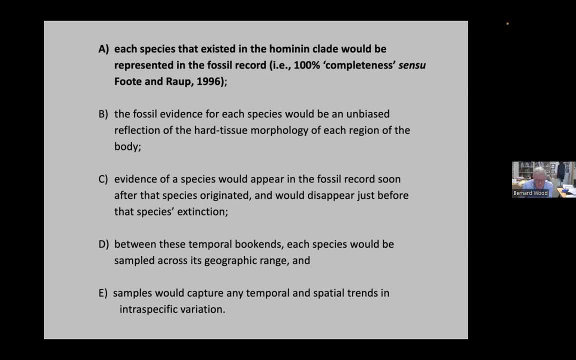 I'm not sure how successful it is. You can be the judge of that. The second part of the thought experiment is that the fossil evidence of each species would be an unbiased reflection of its hard tissue morphology And, you know, hopefully that would be true. 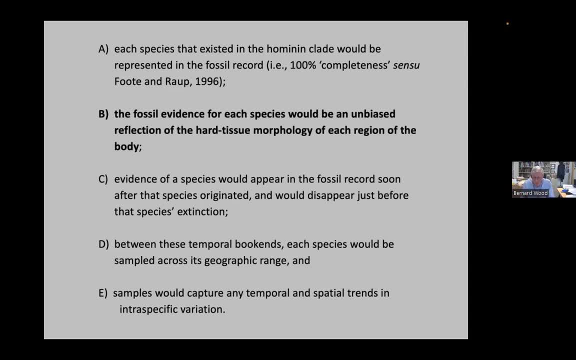 hopefully it would tell us about each of the major regions of the body. The other part of the thought experiment is that evidence of each species would appear in the fossil record soon after that species originated and would disappear just before that species extinction. The next part of the thought experiment is that each species would be 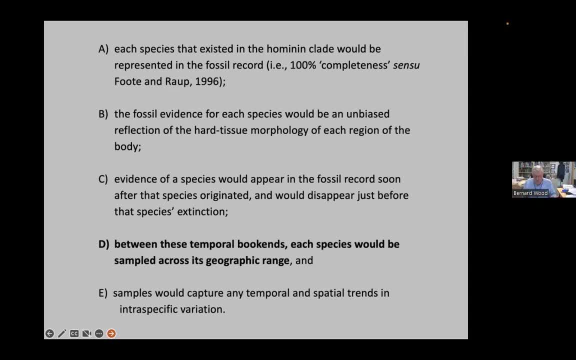 sampled across its geographic range. Now, we don't know what the geographic range of the early hominins that we recognize and you have been taught about, but I'm going to assume in this thought experiment that the fossil record captures the geographic range of each of these species, And I'm also going to assume in the 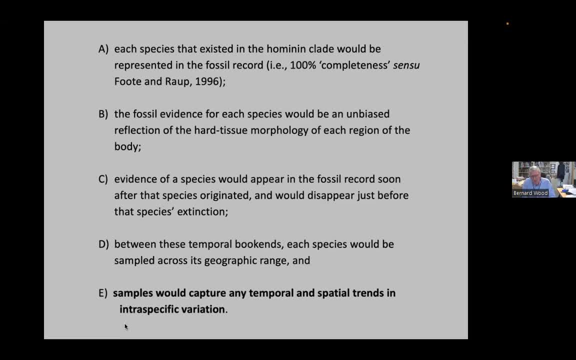 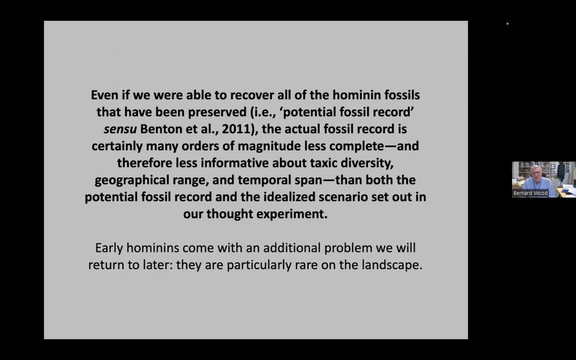 thought experiment that the samples, the fossil samples, would capture any temporal or spatial trends in intra-specific variations. So how far does the existing fossil record differ from my thought experiment? Well, let me sort of come clean, is that I think it would be sensible if we conceded that it probably 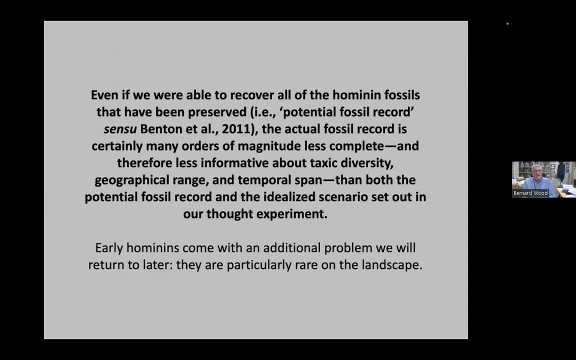 differs quite considerably. Whereas I think there are some people who think that the existing fossil record is much the same as my thought experiment, I think that there is a lot of evidence that the fossil record is much the same And I think that there is a considerable difference between. 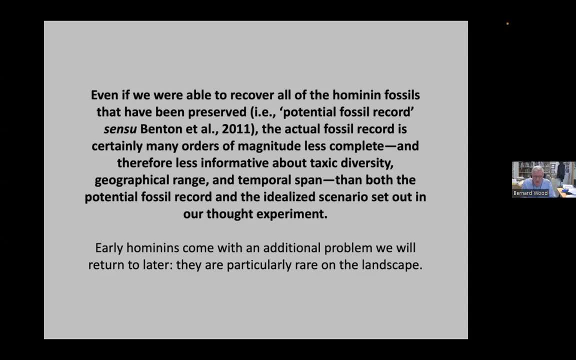 the existing fossil record of my thought experiment. And so even if we were able to recover all the hominin fossils that have ever been preserved- because sort of clearly every hominin doesn't die in a place which is conducive to fossilization- and paleontologists call this the potential fossil record, my sense is the actual fossil record is. 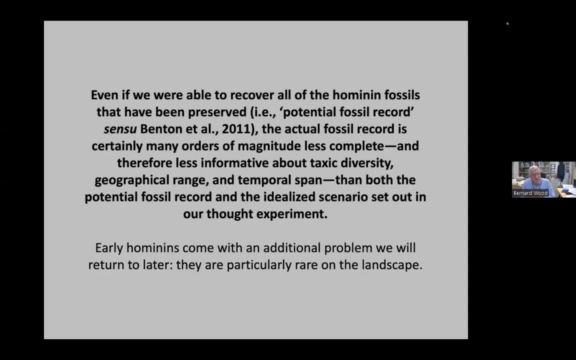 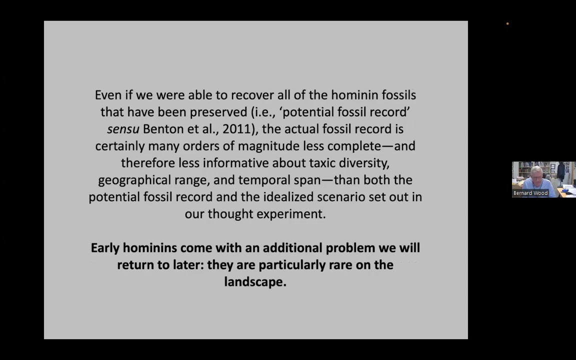 many orders of magnitude less complete And so therefore it's probably less informative about taxic diversity, geographical range and temporal span. And hominins come with an extra problem: that they're particularly rare on the landscape And if you look at hominin sites, there are very different strategies for collecting fossils. 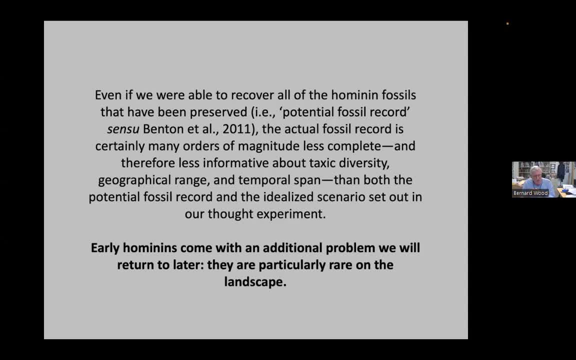 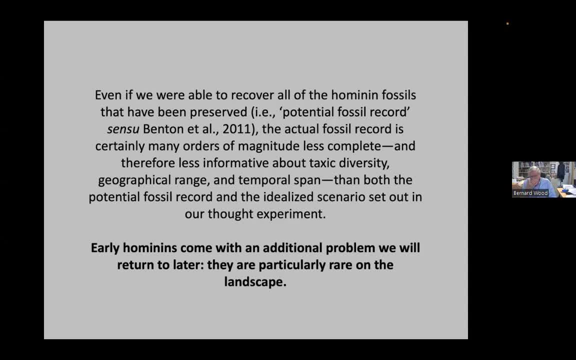 of the mammalian fossil record. So hominins would have been certainly. when I went first went to Kubifora, where the area was just chock full of game. There were herds of zebra, herds of elephants, herds of giraffe and so on. Hominins would have been about as. 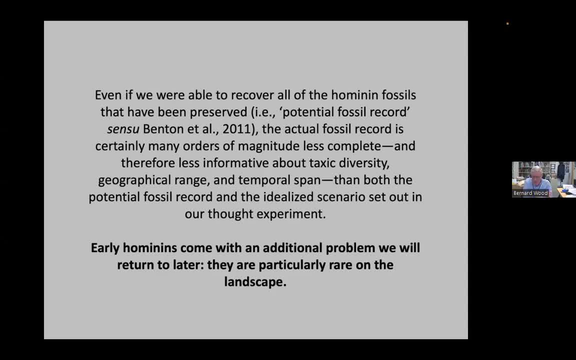 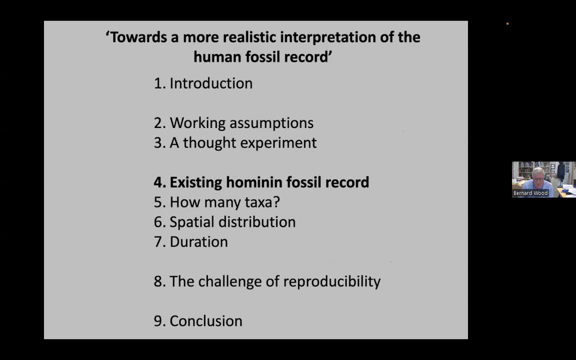 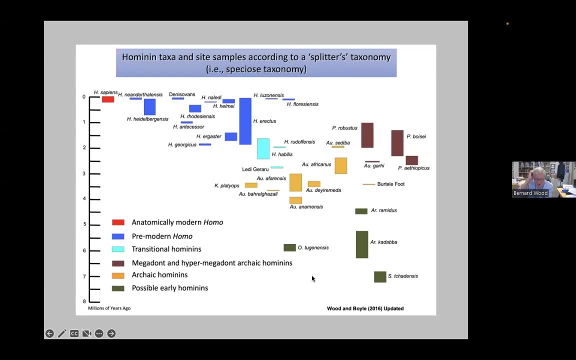 common, as cheetahs were in that scenario, And cheetahs are not very common on the landscape. So what about the existing fossil record? Well, this is a sort of a woodogram of the existing fossil record, And each column is a hypothesis about the existence of a taxon or a collection of 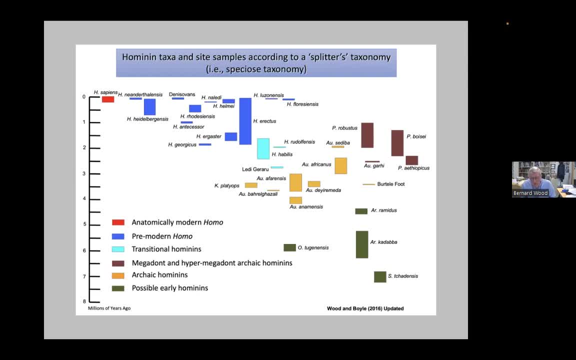 fossils from a site which has not been given a formal taxonomic name. The heights of the columns reflect the distance between the first appearance date, in other words the earliest appearance of a taxon in the fossil record, and its last appearance date. So this is a particularly 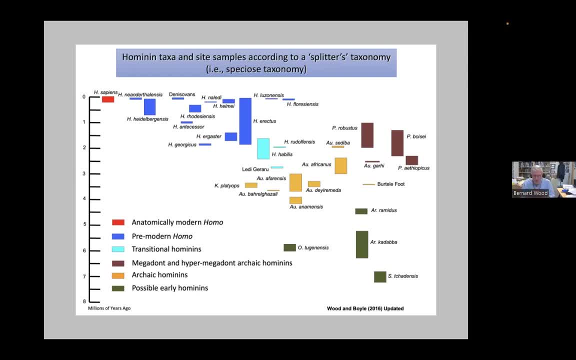 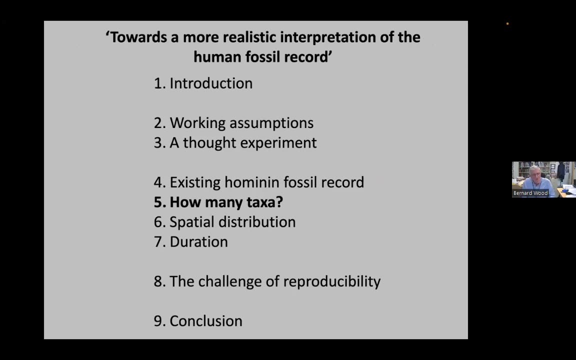 speciose interpretation of the hominin function fossil record. There are people who would interpret the hominin fossil record as consisting of many fewer taxa than this. So if we use that, and we'll use that just for the sake of argument, that is. 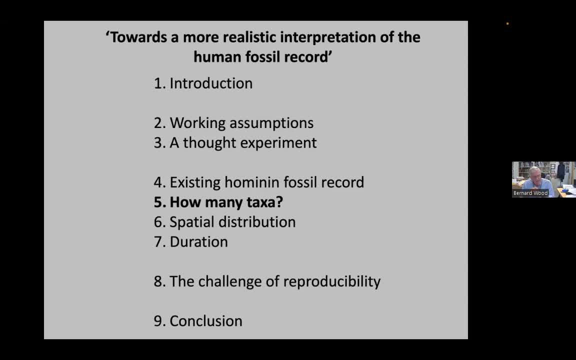 what the existing hominin fossil record looks like. We ask the question: how many taxa should there be, Leaving aside whether you have a tendency to split and therefore to recognize more taxa, or you have a tendency to lump and would recognize fewer inclusive taxa? leaving aside those proclivities, 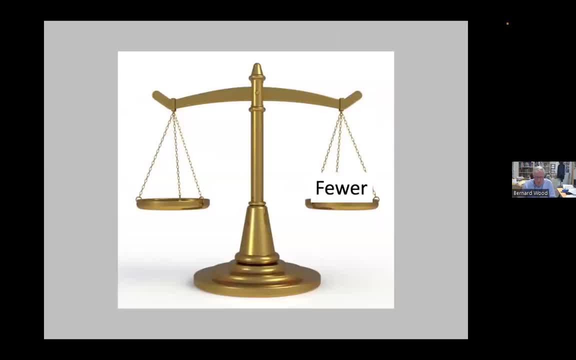 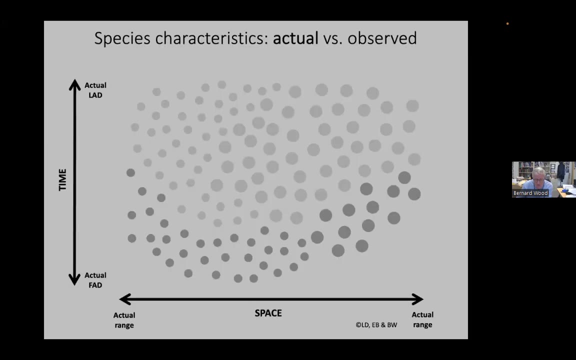 how many taxa should be recognized in the hominin fossil record. Now there are reasons, I think, why there should be fewer taxa recognized in the hominin fossil record, And let me just show you a cartoon, And I apologize, I'm not very good at this sort of thing. 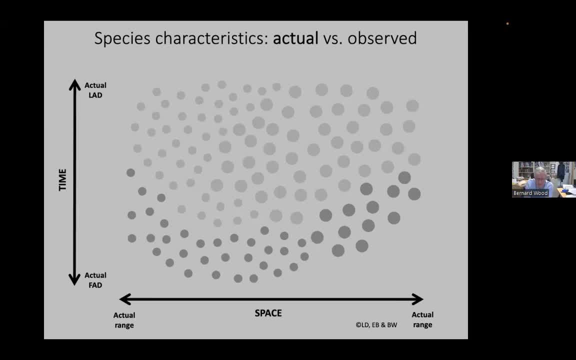 And so this is a pretty hokey diagram. On the left, in the vertical axis, is time, And then the horizontal axis is space. And so here we have a taxon. Its characteristics are gray circles, Some of the circles are smaller, Some of the circles are larger. 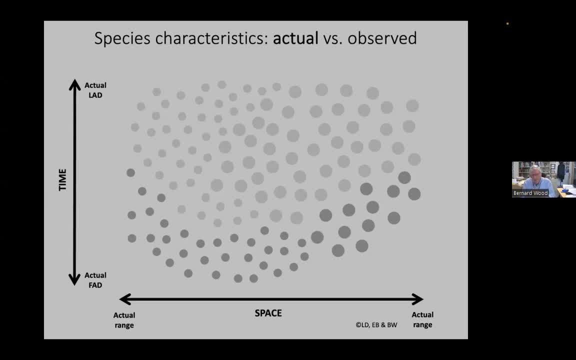 Some of the circles are lighter, Some of the circles are darker, And the point is that this is meant to reflect the fact that, across a million years, which is the average length of a mammalian taxon in the Pleistocene fossil record of Africa, 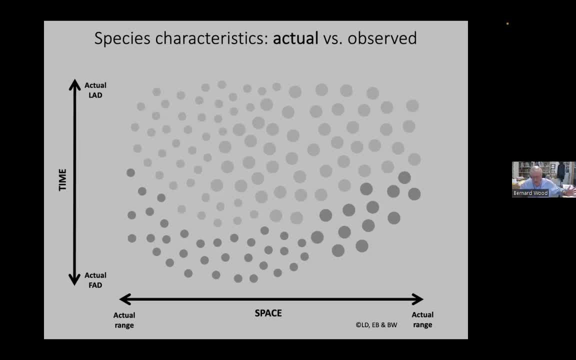 across a million years and across whatever its range was- it could be 1,000 miles or whatever it is. So just imagine on the left is a million years and on the horizontal axis is 1,000 miles. It's the same species. 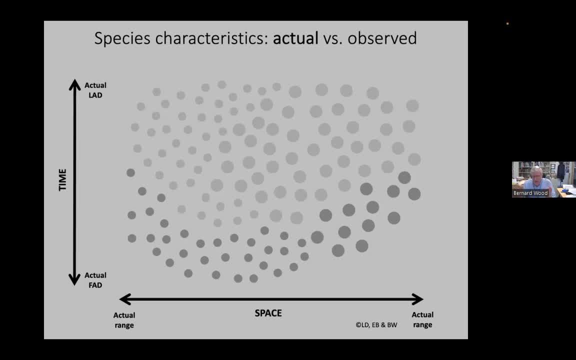 But it doesn't look exactly the same across its range or at different points in time. Sometimes it's smaller, Sometimes it's larger, depending on changes in climate, and so on And so forth. But the thought experiment is that that's a single taxon. 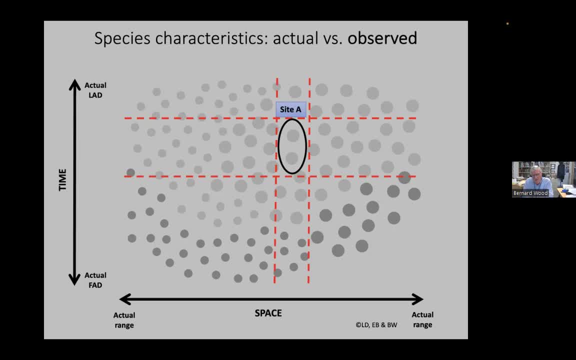 Somebody comes along and they find a fossil site and they find a sample of this taxon, a subsample of this taxon. It's a temporal subsample and it's a spatial subsample And that is large gray circles. 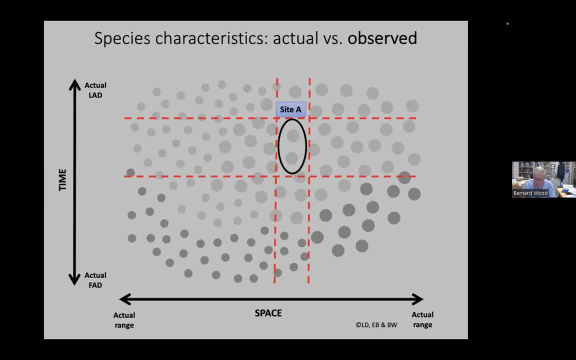 And they write a paper in Nature or Science And they say we found large gray circles. Somebody else comes along a different site earlier in time, much the same region but slightly different region, And they still find large gray circles. 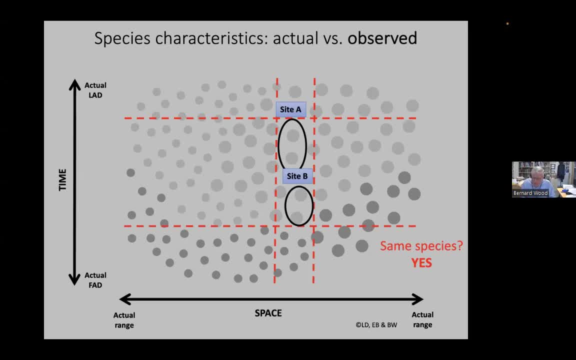 And they don't get their paper in Nature because they haven't found a new species. But they published this in the Journal of Human Evolution. Somebody else comes along. they find a site in a different region. they find large grey circles which we know belong to the same species. 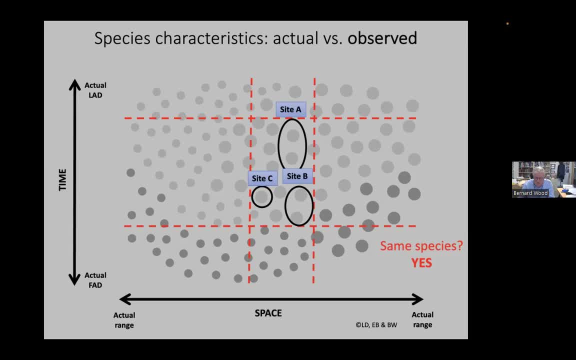 and they publish their paper in the Journal of Human Evolution. Somebody else comes along and they have a slightly different site sample, because they have a mix of large grey circles and small grey circles and they compare the measurements of the teeth or the measurements of the post-cranial bones or the measurements of 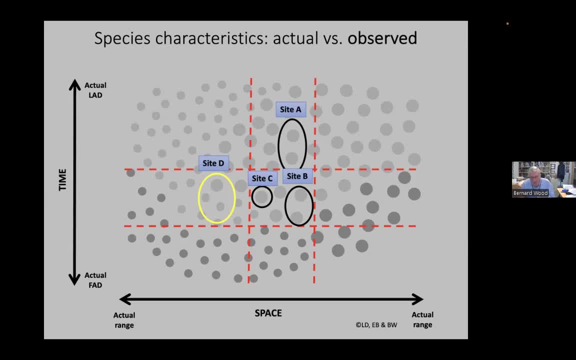 the mandible with the measurements from the site samples from sites A, B and C, and they throw their arms in the air. Boy, we've got something different because our fossils are outside the range of variation of the existing site samples. But you and I know it's the same. 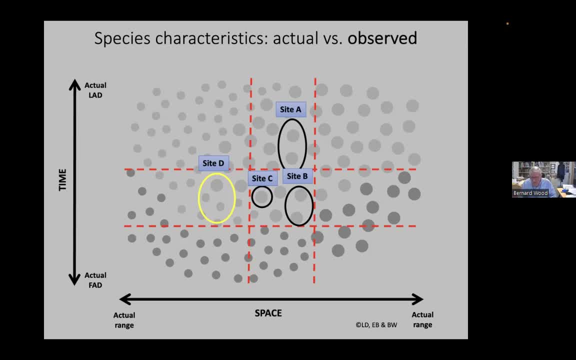 species, But the editors of Nature don't know that, so they accept the paper for publication. So you and I know it's the same species, but the people who find the fossils say no, it's not the same species. And you and I know that the people who find the fossils say, yeah, it's a new species. 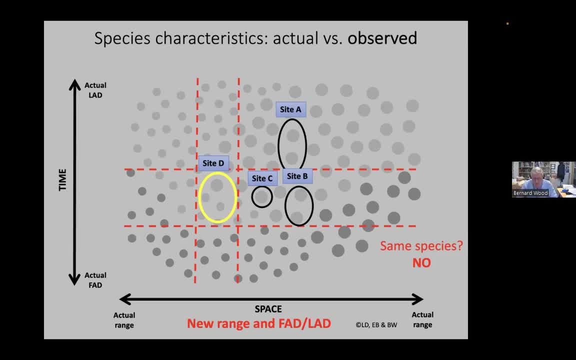 it's got a new range and it's got a new FAD and LAD, But you and I know it's the same species And so that is a reason why the existing fossil record might be more speciose than it actually is, because people have a tendency to say: 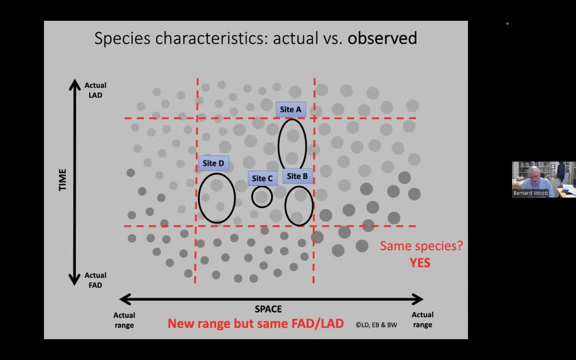 I found a new site. I found a new site sample. It differs from the existing site samples, therefore it's a new species. Well, of course that's not the case. Sometimes that's the case, But in this particular example it's not the case. 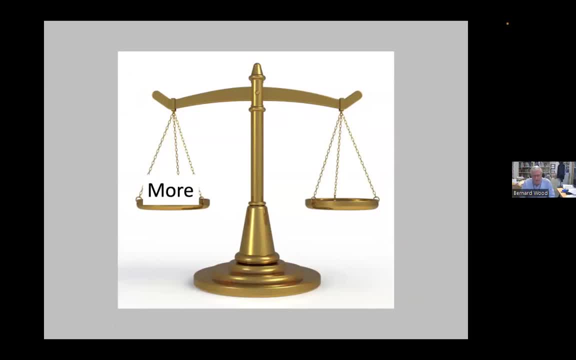 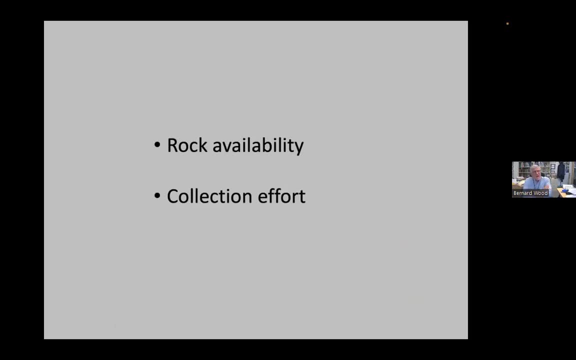 Alan Dulles, might there be more species than are represented in the existing fossil record? Well, there are a whole bunch of reasons why, but one of them was worked on, was written about by Simon Maxwell and Philip Hopley, and they wrote an interesting paper talking about something that other paleontologists 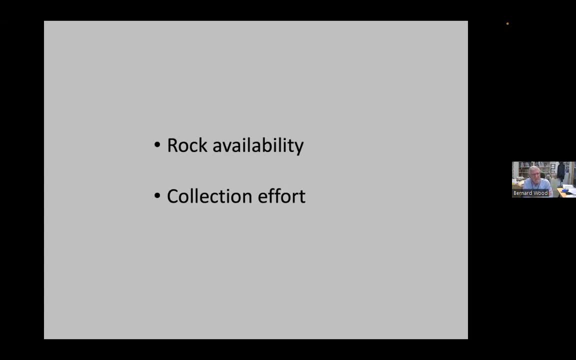 have been talking about for years, which is rock availability. In other words, how, at each stage in time, how much of the sediments that contain the fossils are exposed in a way that would allow those fossils to be recovered. And rock availability is a function of erosion, it's a function of a 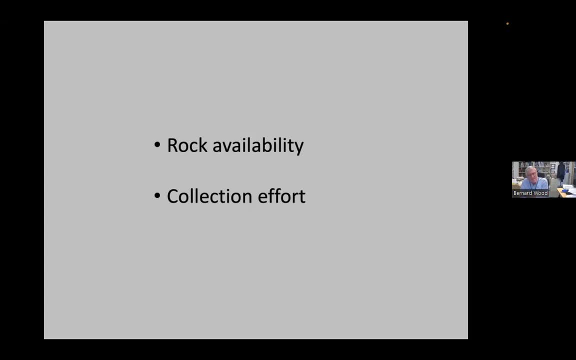 whole band of fossils. it's a function of a whole band of fossils. it's a function of a whole band of fossils And rock availability is highly correlated with collection effort, because clearly you don't make an effort to go and look for fossils if there are no sediments of that. 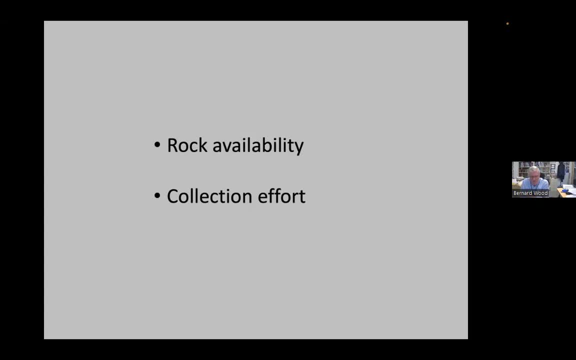 particular time period available in that particular area, And so rock availability and collection effort are a reason why, Although it looks as if some periods there are more fossil hominins than there are at others, the others, the periods when there seem to be fewer fossil hominins, may be times when there is. 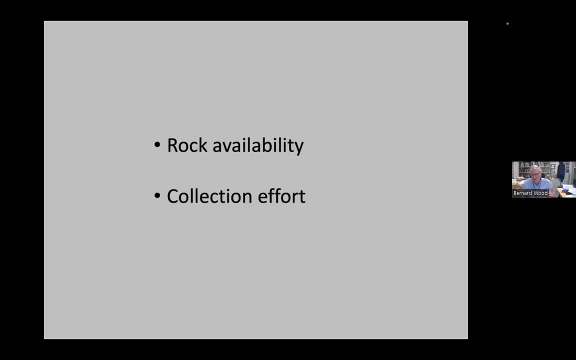 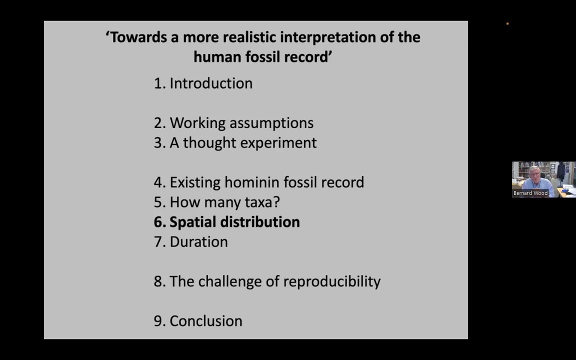 not as much rock available to look for fossils and therefore not as much effort has been made to look for fossils, And so those are just two of a bunch of reasons why the existing fossil record may not reflect the taxic diversity in the hominin claim. The next thing. I just want to spend a couple of minutes. 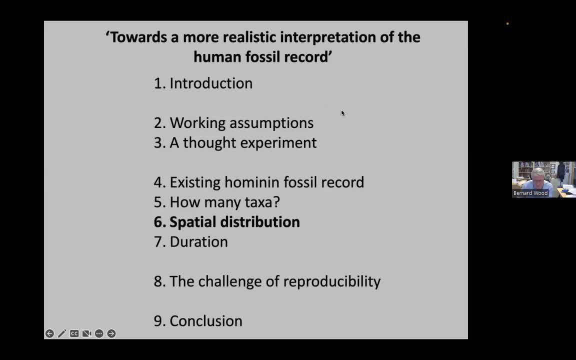 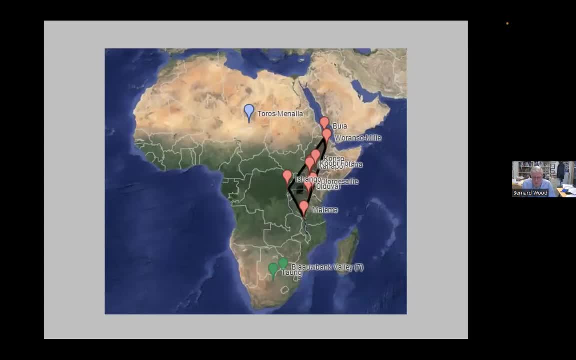 talking about is spatial distribution, And if you plot where hominins are found in Africa, it's basically in two. There are sort of two windows that are provided in Africa. One is the window which is provided by the East African rift system and the sites that are either in the rift or around the rift. The other window is an 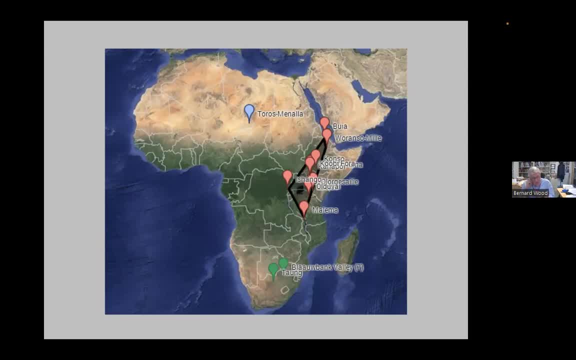 even smaller window, which is the cave sites in the Dolomitic uplands of Southern Africa, And there are a few. There are a few early hominin fossil sites, not in those two regions. One is in Chad and there are a group of localities in Chad. Now there are other places where hominins have been found in Africa. 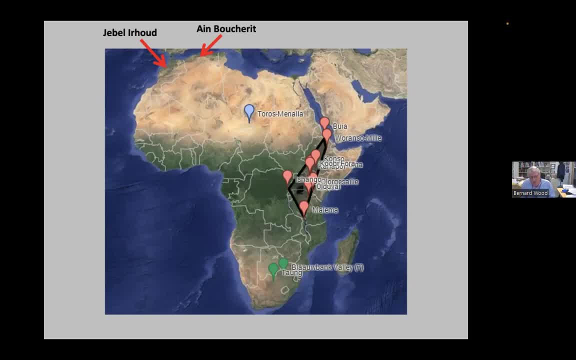 and Northern Africa, but not early hominins. So if you add all these places together, the area where there is rock availability, that people have committed collection effort and therefore have found hominins, probably represents between two and three percent of the land surface of Africa. 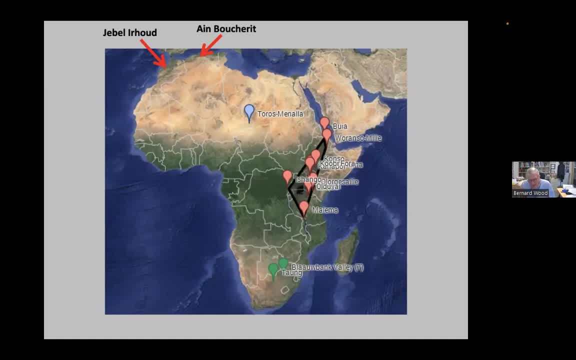 Now, and these places are like lampposts. you know They are. You can imagine Africa being this huge parking lot. Africa is a big continent. It's three times the size of the United States. It's a big continent. 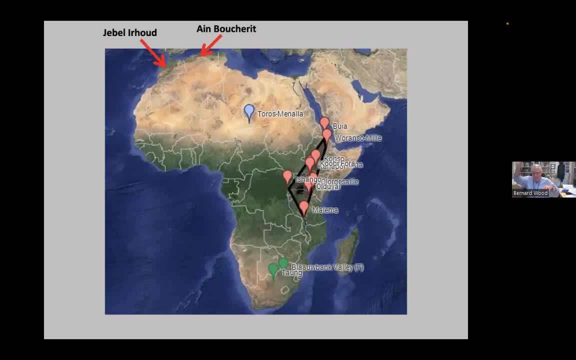 But you can imagine Africa as this huge parking lot And in this huge parking lot there are two lampposts where you can see underneath the lamppost, And these represent the areas where there are fossil sites. And this person comes back from the city worse for wear, having been to a dinner. 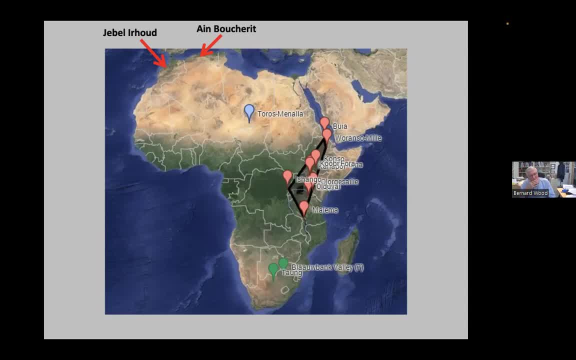 and she or he gets their keys out as they come from the train, And somewhere between getting their keys out as they got from the train and getting to their car, they drop their keys. Now where do they look for them? Well, they look for them under the lampposts. 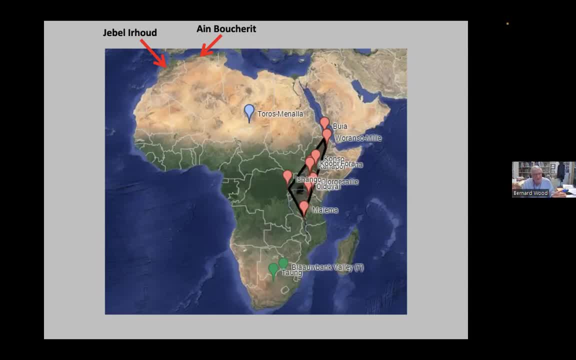 It's the only place you can see, Otherwise you're going to have to crawl around on your hands and knees trying to see if you can feel your keys, because you can't see. So these two regions are a little like you know, the lampposts under which the drunk looks for their keys. It's the only place. 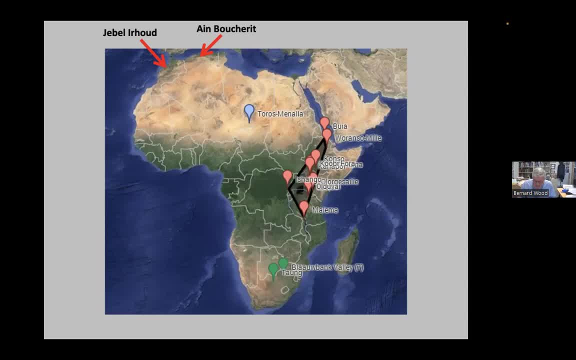 you can look, But does that mean that's where the keys are? Probably not. And does that mean that all significant events in hominid evolution either were played out in these two regions or were captured by evidence from those two regions? And I think that is just a? 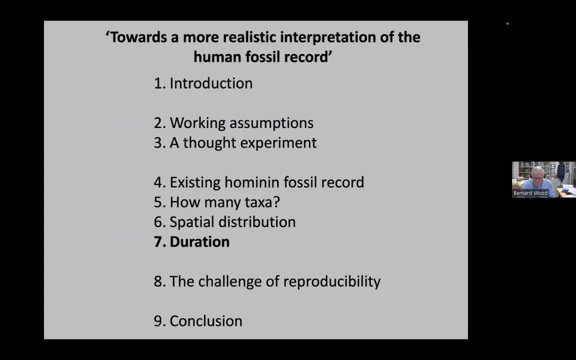 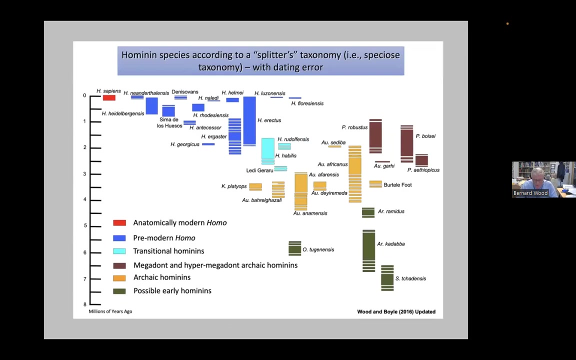 crazily unlikely scenario. So what about the time? And the thought experiment said that you know, the hominins would, there would be a fossil record soon after they appeared and the fossil record would end just before they became extinct. We know that, that is, we know that these columns 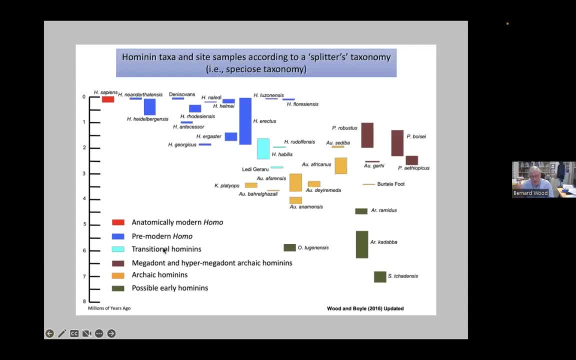 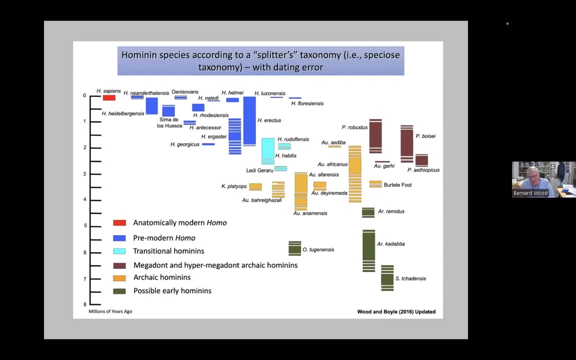 let me go back. we know that these columns are minima. Okay, It's likely that hominins were around before the first appearance date and it's likely that they were around after the last appearance date. There are various ways in which you can try and estimate the confidence. 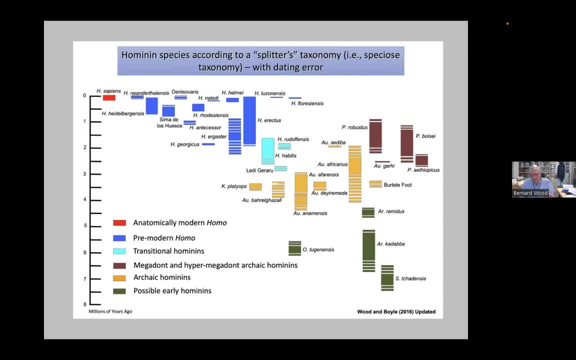 intervals of the first and last appearance date, And they depend on you know. for example, are there any fossil sites where there are no hominins that predate the first appearance date of, say, Australopithecus afarensis? And you then have to say, well, what does no hominins mean? 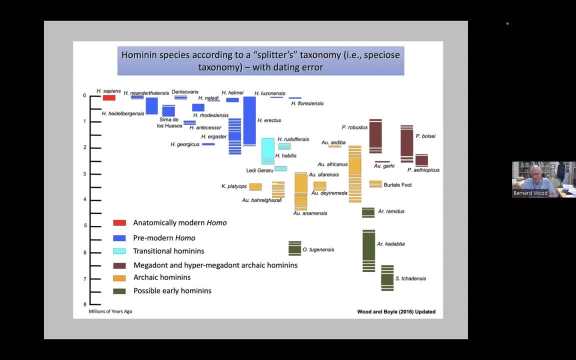 Well, no hominins means probably that you have to find several hundred bovid fossils or several hundred pig fossils before you can begin to think that there were no hominins, Because hominins are so uncommon: just finding a few mammalian fossils, but not finding hominins. 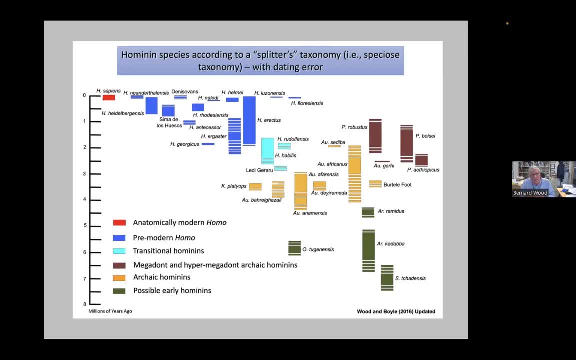 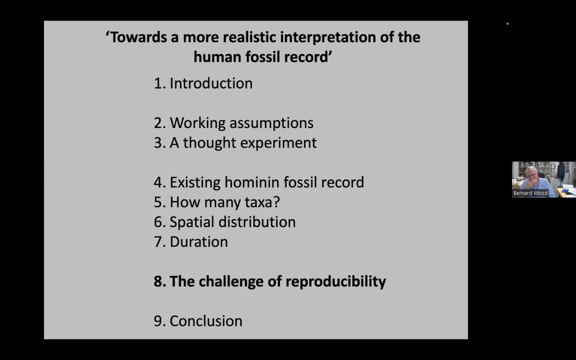 does not mean that hominins were not there, And so hominins are a really, you know, a good case of absence, of absence of evidence is not evidence of absence. Then there is the challenge of reproducibility, And the thing is, and I've done this myself, and so 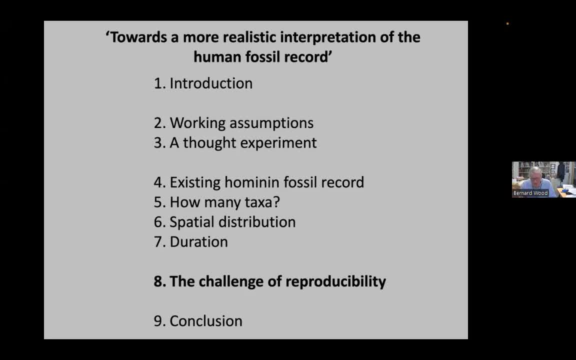 nearly all my comments are as directed against me as they are as anybody else. The question is: what methodology do you use to interrogate your fossil record to work out whether you think there is evidence to recognize a new taxon? And the answer is: you obviously can only use 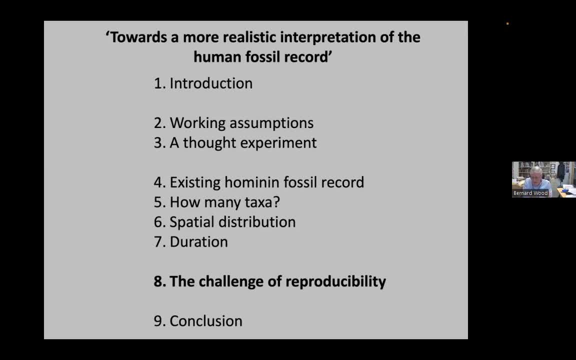 the evidence that you have. In other words, if you only have teeth and jaws, then you have to do it on the basis of teeth and jaws, But if you and the evidence that you have may not be the evidence you would like, because it may not include areas that are likely to be, 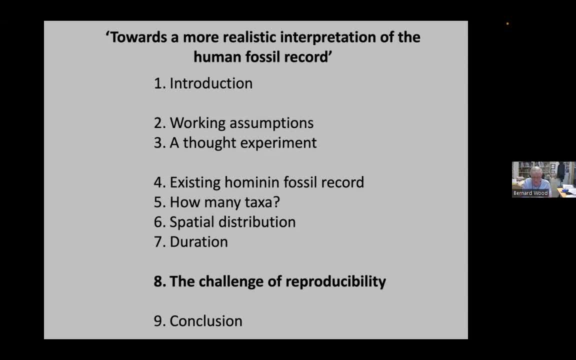 sensitive to taxonomic distinctiveness. And the other thing is that there are confirmation biases going on the whole time. There are sort of there are cognitive biases, I'm sorry, of which confirmation bias is one? And although as individuals we say well, I'm not biased. 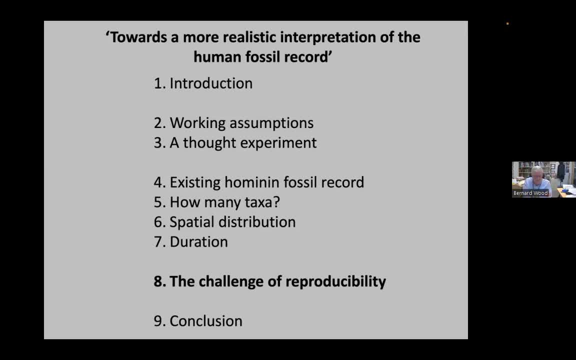 I go about this. I have no, you know, I have no preconceptions. That's just not true, apparently. I mean, you know as much as we would like to think, it's just not true. And so, when you add all these problems to how we should view the existing fossil record, 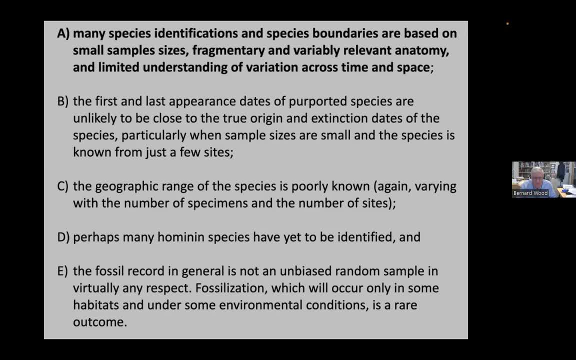 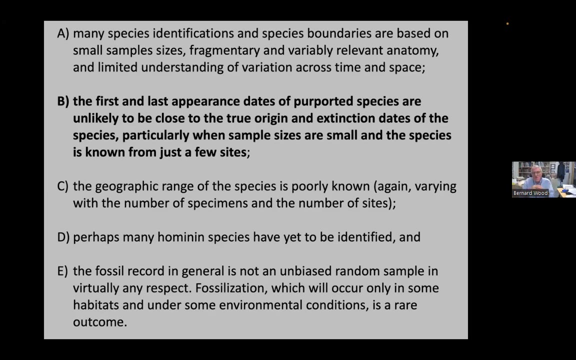 my sense is that we probably the existing fossil record gives us a very limited sense of what the actual fossil record was, For various reasons. the locations of those columns, those columns are all likely to be taller than they actually are, And this kind of applies to, you know, other kinds of fashion. 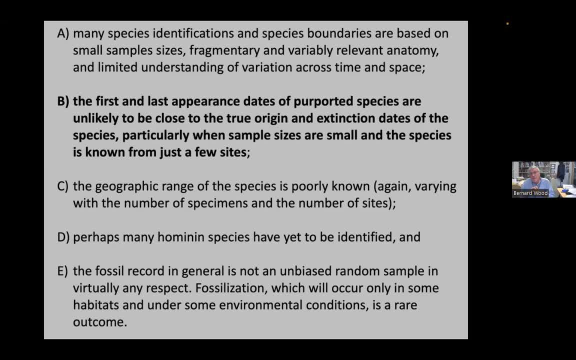 And this means that if any of those columns line up on the existing fossil record, it's a fool's errand to try and sort of chase some explanation, Because those columns are not when attacks are revolved or when they became extinct, They are minimal. 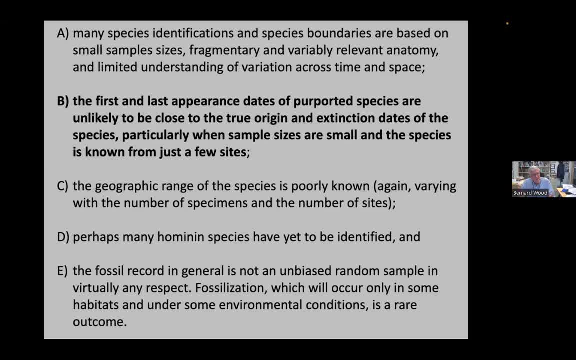 And so you know, if you try and sort of chase some sort of climatic explanation for something that happened at 1.8 million years ago, it probably didn't happen at 1.8 million years ago, It happened before 1.8 million years ago or it happened after 1.8 million years ago. 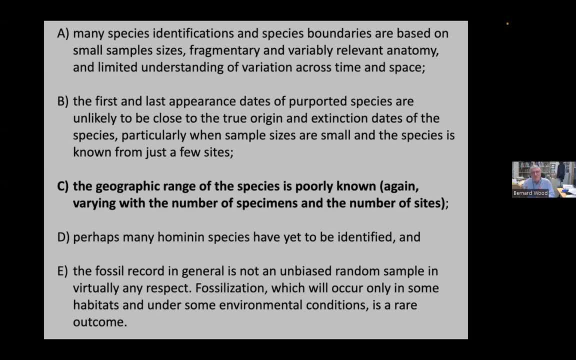 My sense is that, unless you think that hominins were confined to the East African rift And to the area the Dolomite in Southern Africa, that we have a very poor sense of what the geographic range of hominin species was, And because hominins are so rare, it's likely that there are several, if not many, hominin species that have yet to be identified. 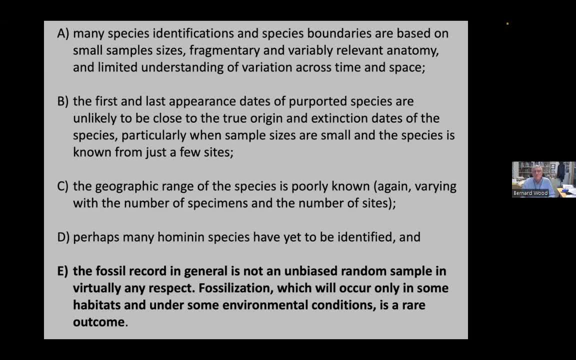 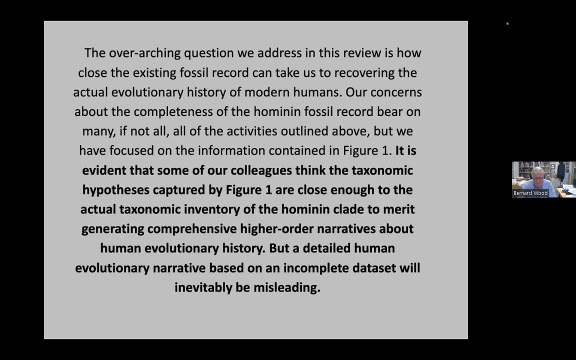 And Fossilization will occur in some paleoenvironmental conditions and not others, And therefore this is another reason why the existing fossil record is likely to be misleading. But it's pretty evident that some of our colleagues, some of my colleagues, think that the taxonomic hypotheses captured by the figure 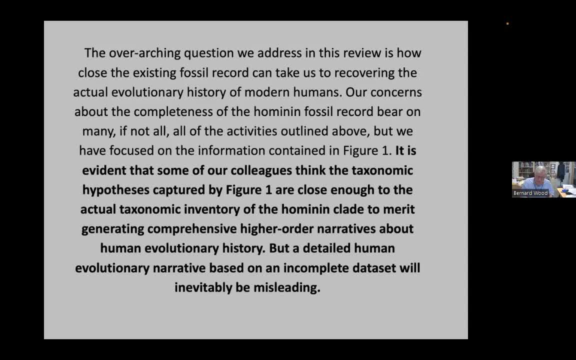 Are close enough to the actual taxonomic inventory of the hominin clade to merit generating comprehensive, higher order narratives about human evolutionary history. But the problem is that if you come up with complex explanations for an incomplete data set, they're almost bound to be wrong. 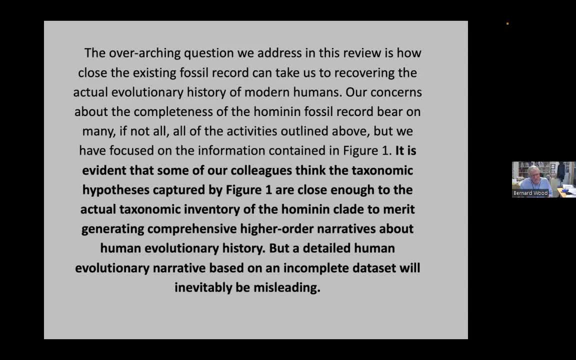 And And. Although we each of us have an urge to do this, we need- even if we can't resist the urge, we need when we are giving into the urge, we need to have a little person sort of sitting on our shoulder, just saying: just want to tell you that this might be a fool's errand. 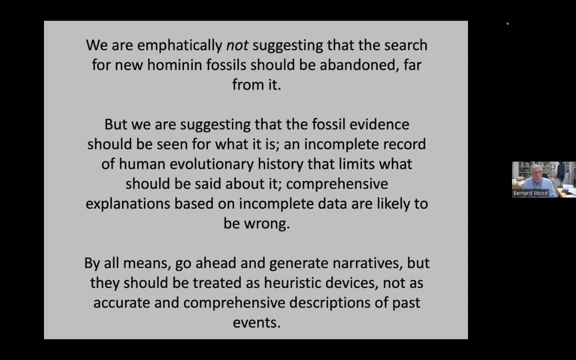 So We're emphatically not Suggesting that you know that, that that all is lost and there's no point in looking for hominin fossils. That's, that's ridiculous. But we are suggesting that the fossil record should be seen for what it is, which is an incomplete record of human evolutionary history. that limits what should be said about it. 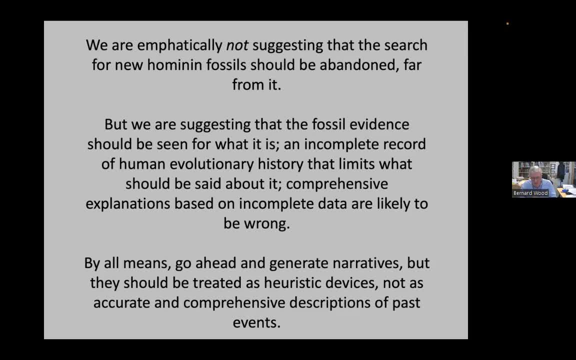 Comprehensive. explanations based on incomplete data are likely to be wrong And by all means go ahead and generate Narratives, but the narrative should be sort of treated as heuristic devices, not as accurate and comprehensive descriptions of past events. And the other thing is, you know, I mean, I've been wrong so many times that that that that you know, I've had to get used to it. 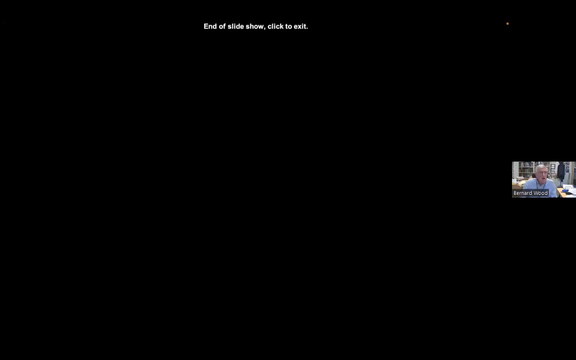 I, I would urge people, even if you think that this paper and this presentation is not really accurate, I, I would urge people, even if you think that this paper and this presentation is, is, is, you know, might contain some hype, some hyperbole, I would urge you to at least give some thought to what I've said, because if you don't, I think you're going to waste your time coming up with explanations for things that actually don't exist. 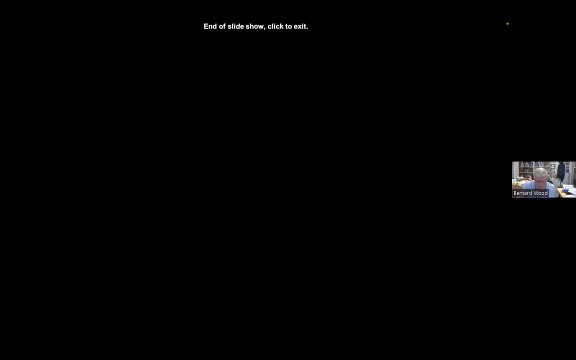 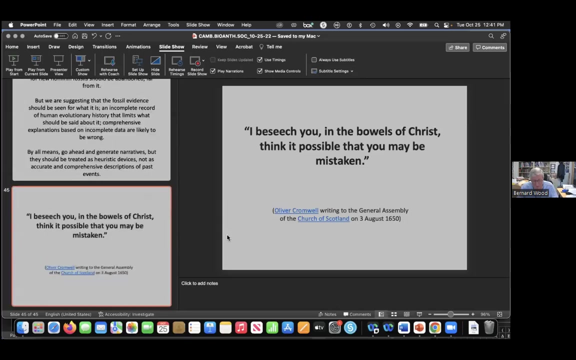 So thank you for allowing me to speak. Thank you for allowing me to talk that long. My screen is now blank, but I'm assuming that I can do something about that. Let me escape, Okay. Oh, the last one. David filming sent me this quote from Cromwell: 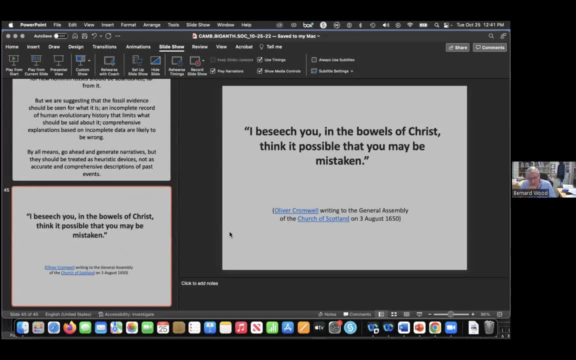 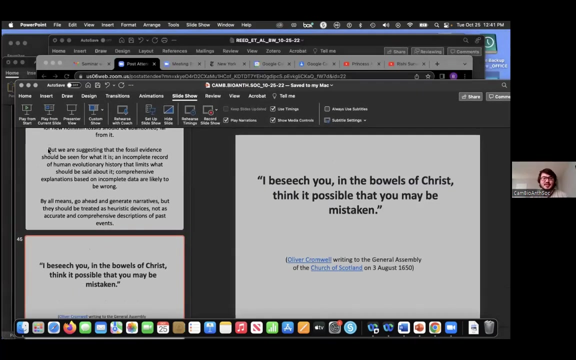 I beseech you in the bowels of Christ. I think it possible that you may be mistaken. That's my parting message, Thank you. That's the word for this, this presentation, and we'll now go ahead and open it up to a Q&A session where you can either raise your hand or submit a question to Dylan or I, and we'll read it out for you. 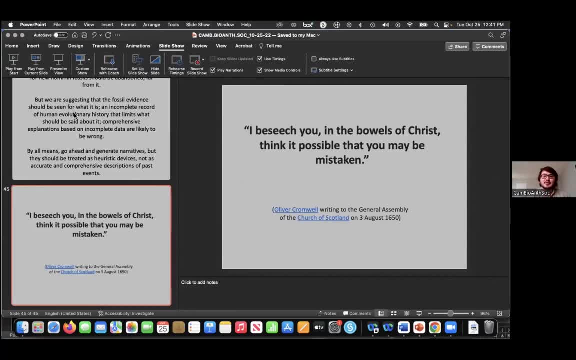 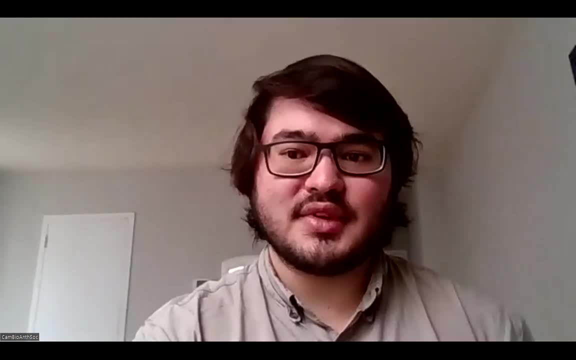 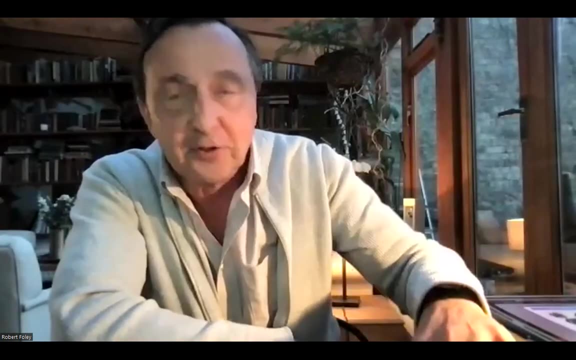 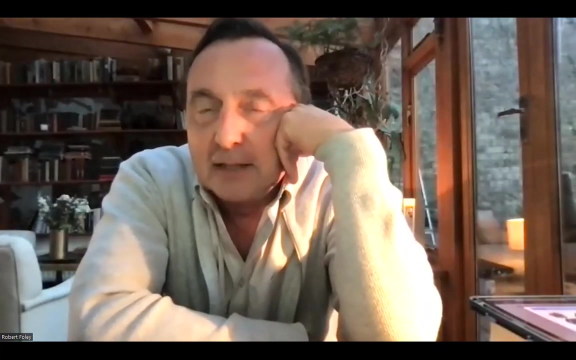 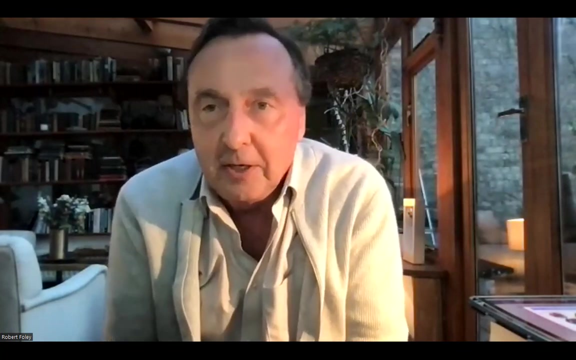 I'll, if you like, I'll. Bernard, I'll start off. How are you? Nice to hear you, Nice to see you? Can I say that wasn't the most cheerful talk on human evolution I've ever heard, Particularly if we had- we had Lee last, last week, who is, is, is, is Tigger to your EO, I think. 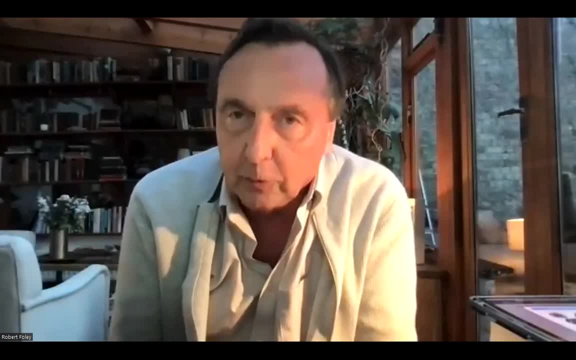 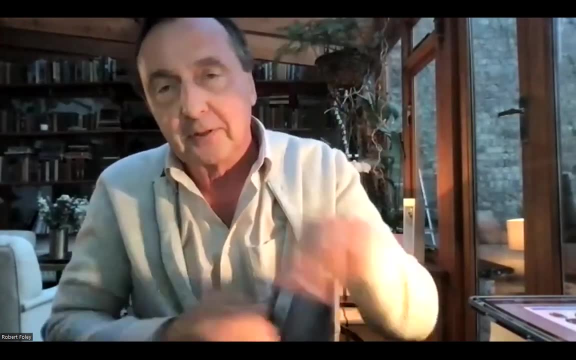 I mean, I take your point and we have to be very cautious, and I'm probably one of the people you had in mind when you, you know, talk about trying to sort of build models and things of grand nature. But take your point. 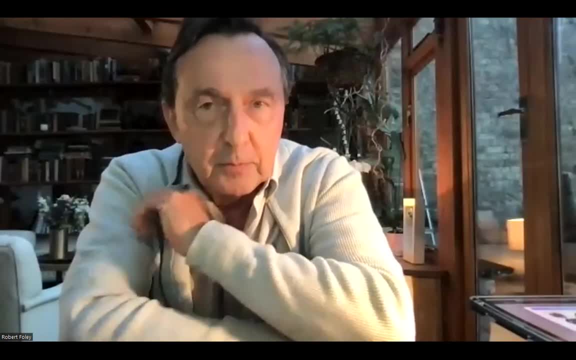 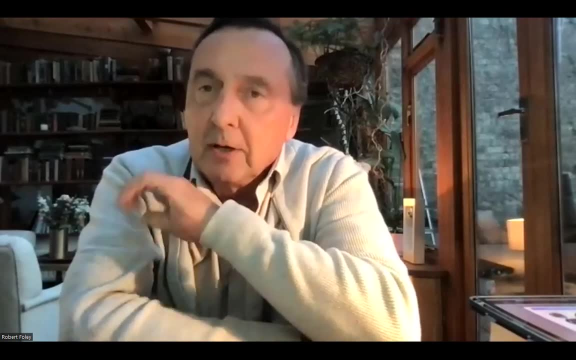 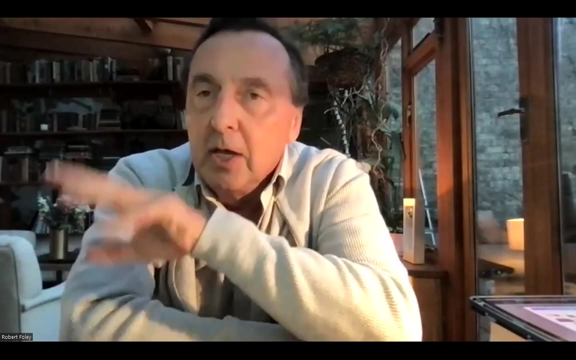 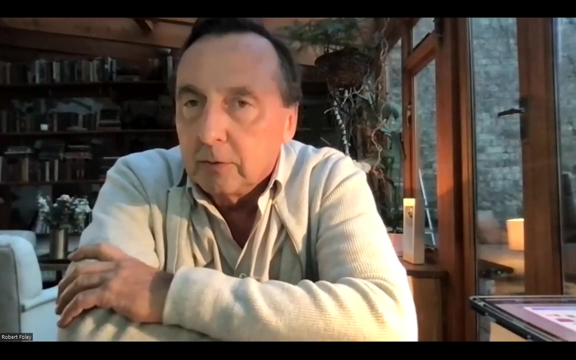 You know, okay, let's let's keep away from macroevolutionary questions. but my, then what if you were to advise students starting out? what should they questions, should they be asking you? you think you can get secure answers because you're suggesting we can't get them on the macroevolutionary patterns. but there must be a core area where you think, okay, this is a more reasonable set of questions to approach. 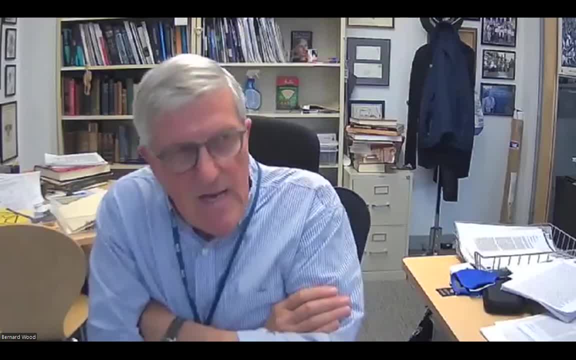 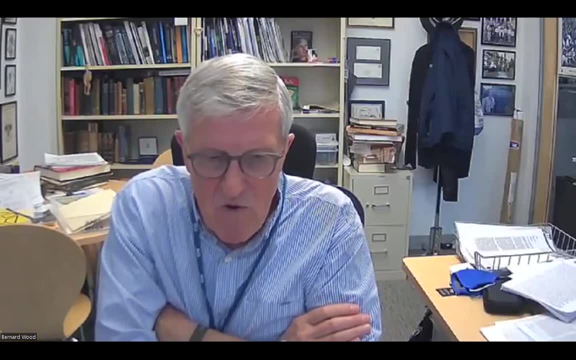 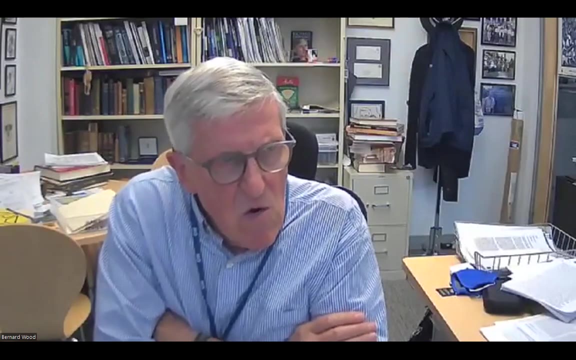 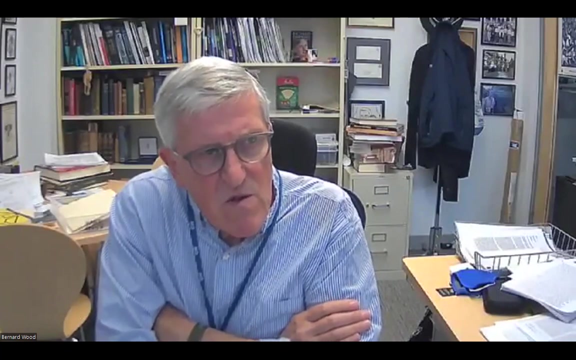 Well, I think you know, trying to work on How many taxa you know would be a very sensible thing to to pursue, but it would be. So you know how do we go about working out whether a collection of hominin fossils is so variable that it it is highly unlikely to sample just a single taxa? 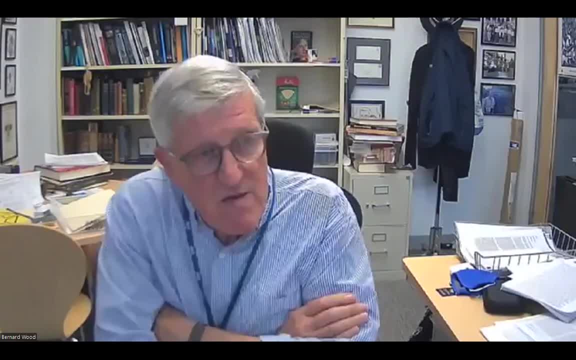 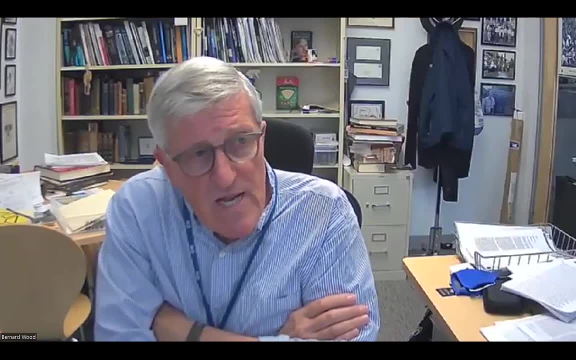 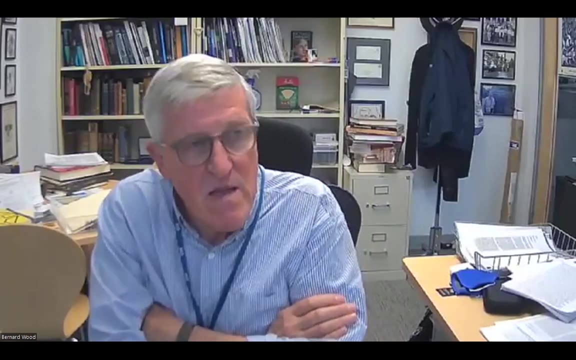 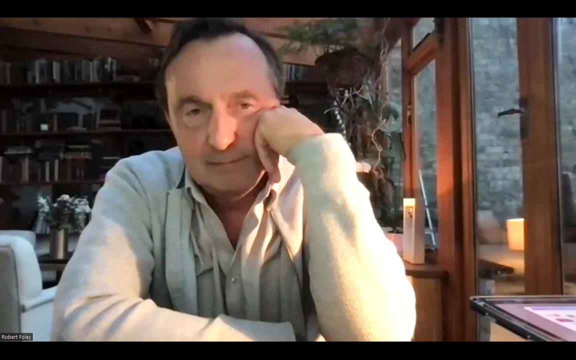 The problem is, you know that our extent models Are either modern humans or they are closely related, higher primates which lack the distinction of hominins, which is having small canines, which you know. I'm not saying that every higher primate with small canines is a hominin, but to be a hominin you probably have to have small canines. 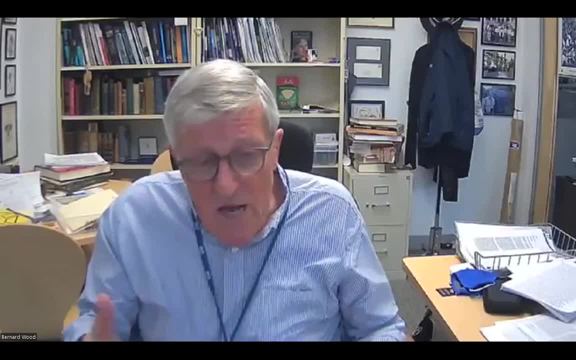 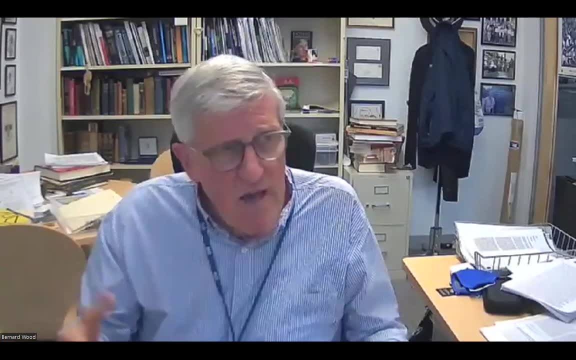 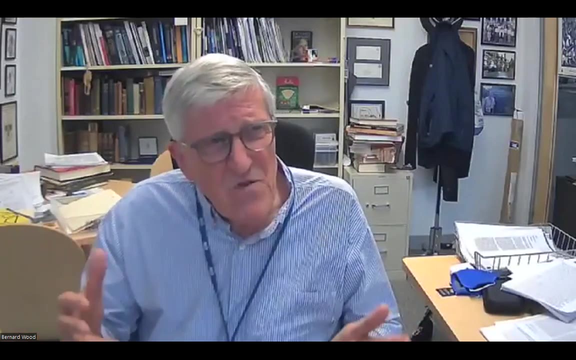 And so so we don't have a comparative model And the comparative Models you know, even if we accept that sort of chimpanzees and bonobos, are a good comparative model. Most Collections of chimpanzees and bonobos in museums. 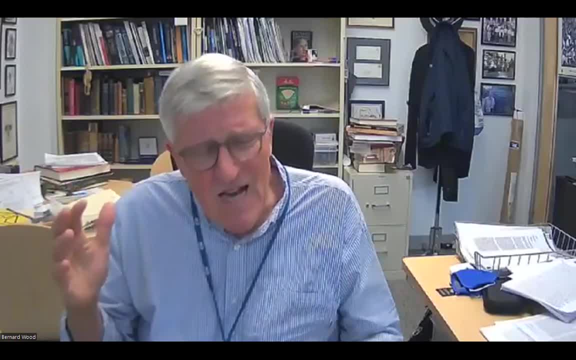 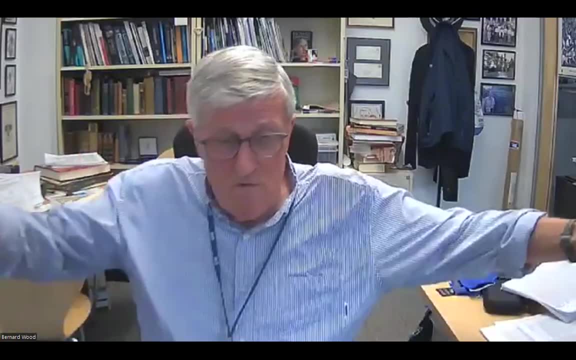 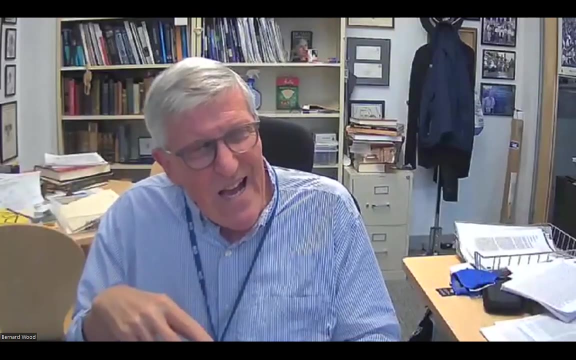 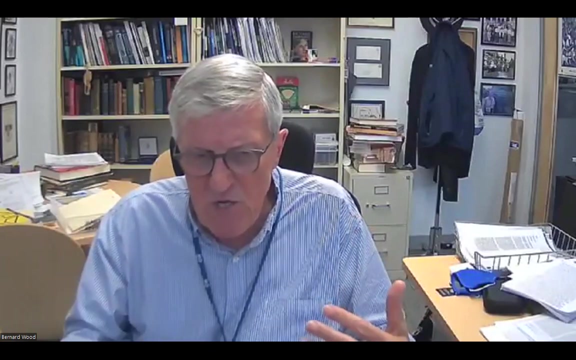 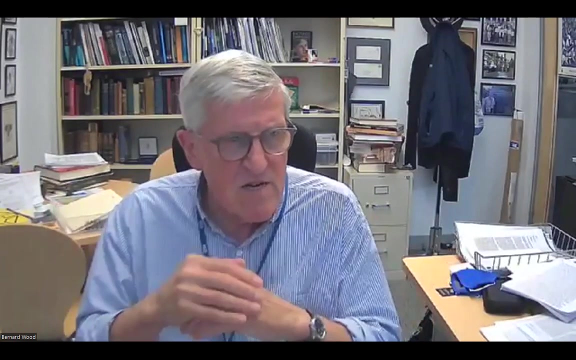 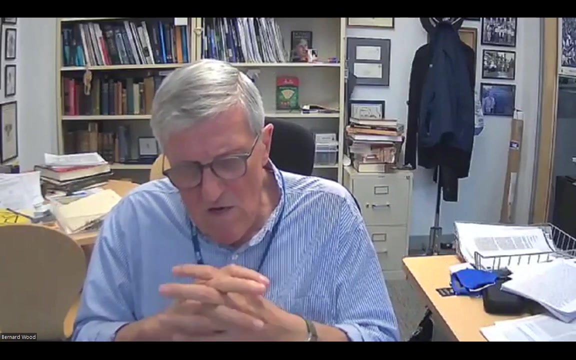 At the moment, you know, the most span 100 or 150 years of time And they come from a single location or, you know, if not single locations, they come from the same region. So how do we translate that into into a yardstick for making judgments about taxonomic heterogeneity? and that is something that I've been thinking about for the whole of my career and I have not come up with a satisfactory solution, and I'm just hoping that, you know, a bunch of smart people will come along with a satisfactory solution. but I mean, you know, I'm not sure what it is. 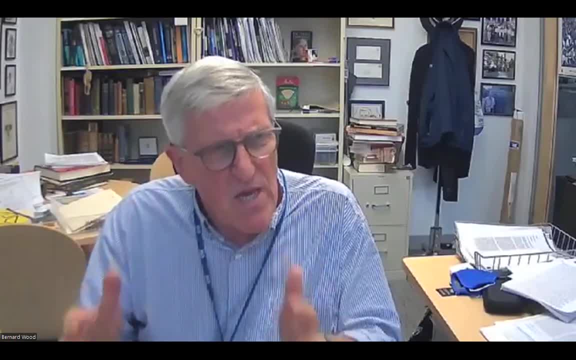 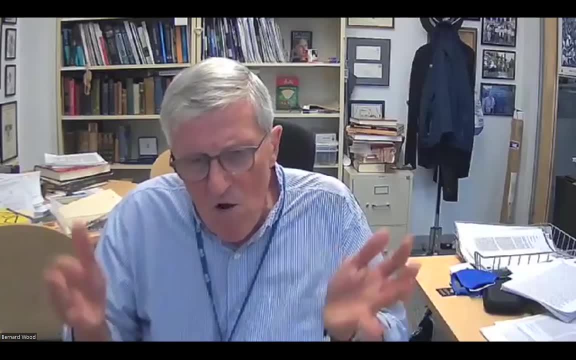 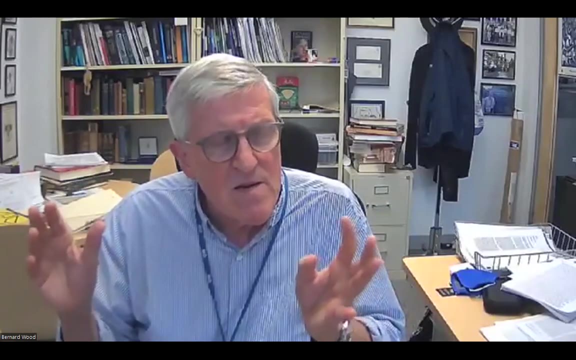 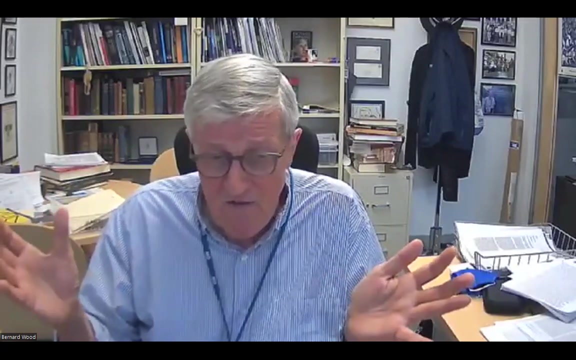 So, So, So I think there are lots of interesting things to ask. you know, what were these creatures doing? how are they moving around, what was their posture and what were they eating? All those are reasonably tractable questions. but you know, why did hominins become bipedal is a really attractive question, but it's not a question that I think you can answer scientifically. 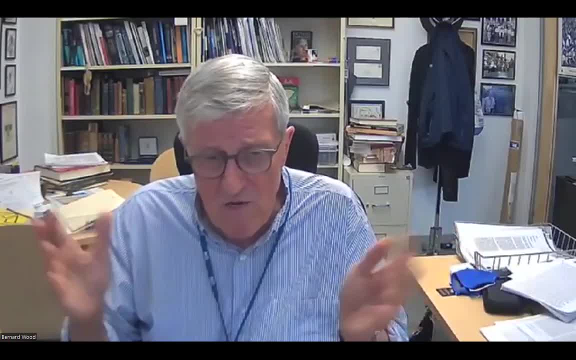 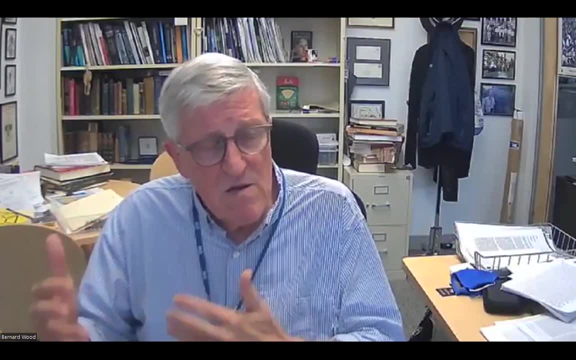 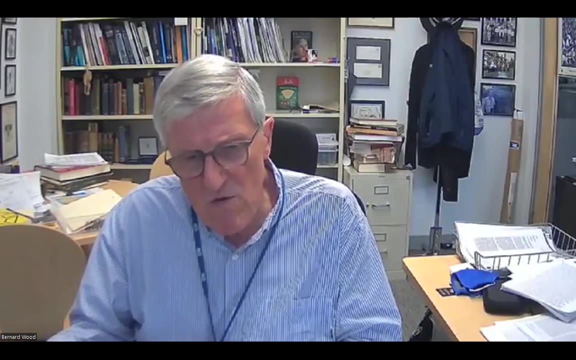 In the absence of a time machine, I don't think you can answer it scientifically. So I think you know the The. The answer is: try and tackle questions that can be answered scientifically and try and stay away from questions that mean that you have to stray away from science in order to answer them. 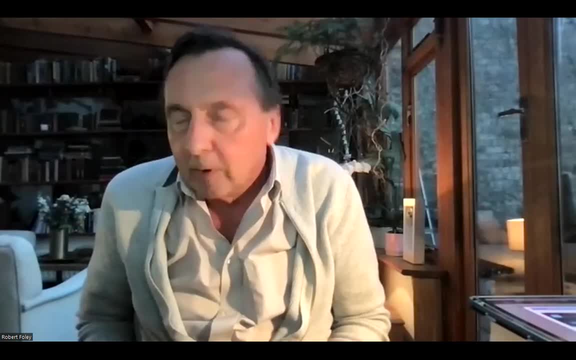 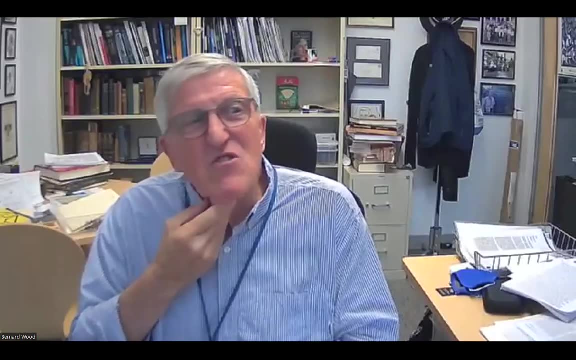 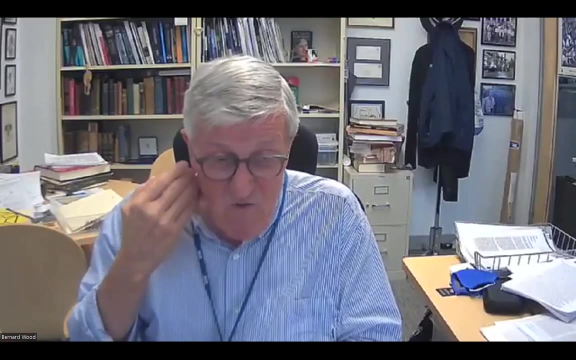 So I mean just to follow up in a way. you're saying paleoanthropology should get back to its functional morphology roots. Well, I'm saying paleoanthropology should function like other branches of paleontology Which Tend not to answer. 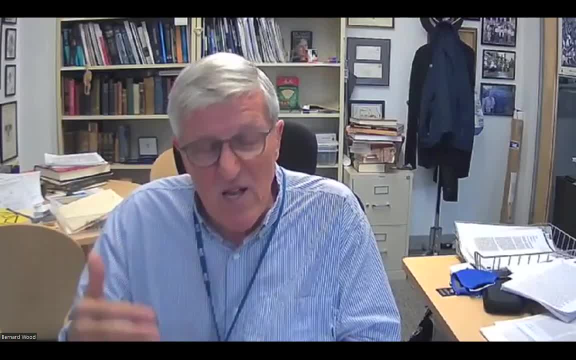 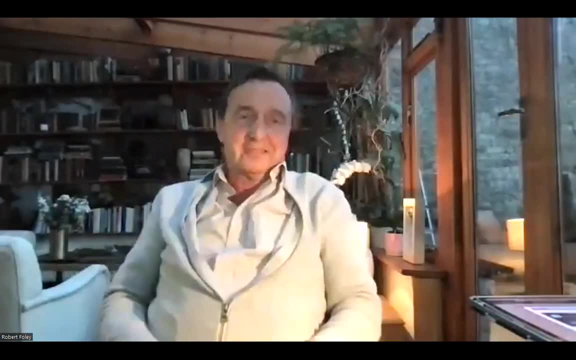 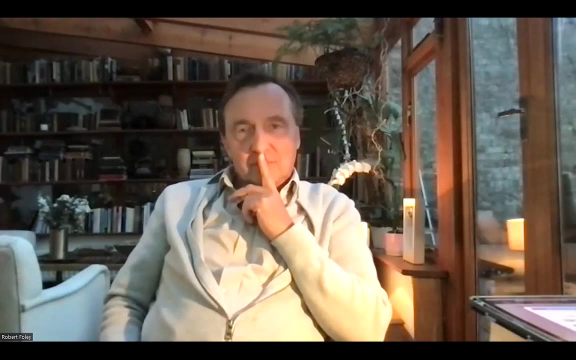 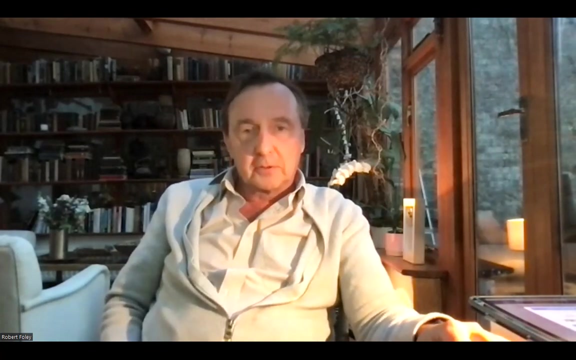 Which Which tend Not to ask why questions? Hmm, I will, I will think about that one. Thank you. What should I agree with that? But anyway, thank you very much. I Think there's a. there's a question that Dylan flicker wants to ask. 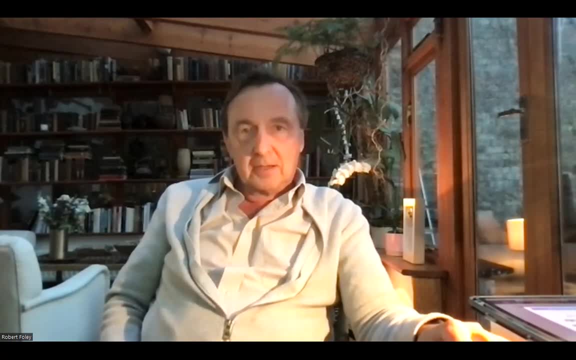 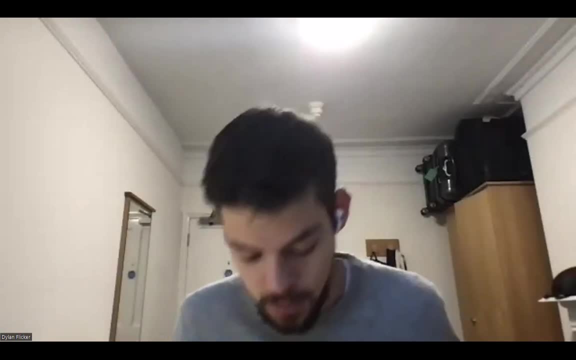 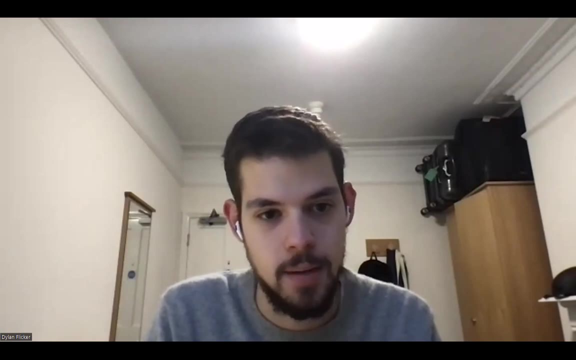 Who Probably just yep. uh, so sorry, it seems like jared's like wasn't quite working there if he was calling on me, but i do have a question which is, uh, related to why you prefer a species taxonomy, as was displayed during the talk. um, you mentioned that the reason for preferring to interpret the fossil. 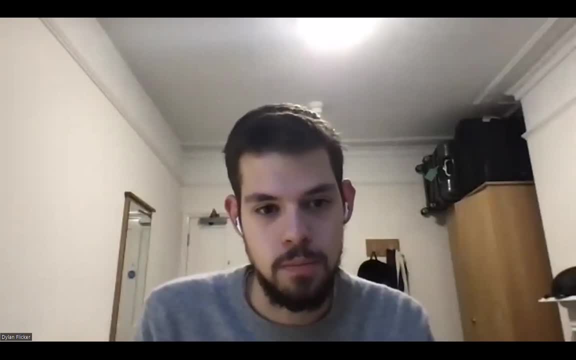 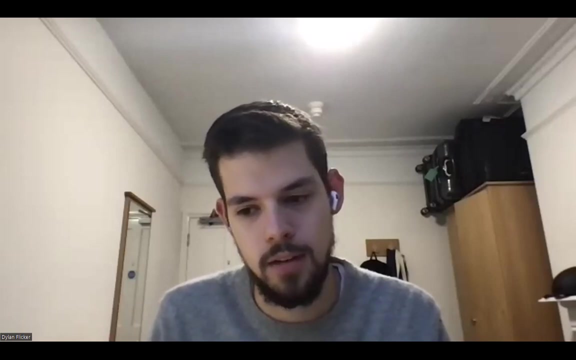 record with more interspecies. variation would be because of the sampling method across space and time with which paleoanthropologists must recover fossils um, and that the reason for preferring a species taxonomy would be that we don't really know the full diversity of um of taxa in the past. because we haven't recovered all taxa because of rock availability and collection effort. it seems like the reason to prefer more interest in the fossil record is that we have recovered more than we have recovered, so the specific variation would be based on the observance of what we have currently recovered. 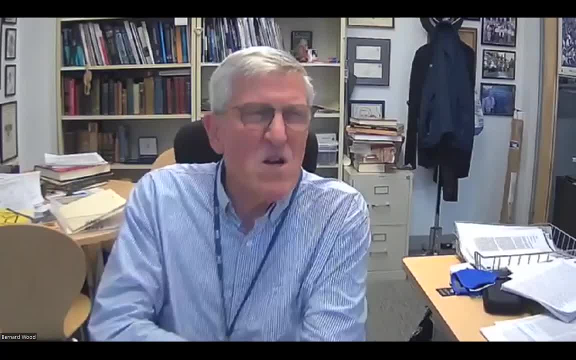 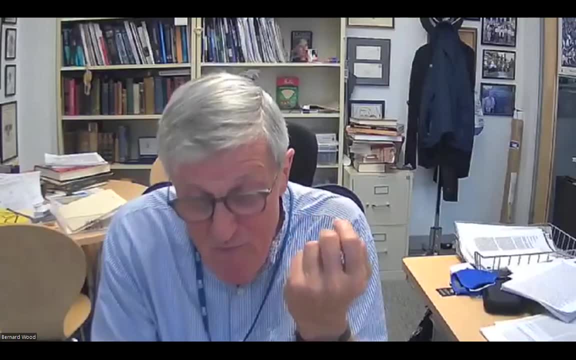 whereas we wouldn't prefer a speciose version of the fossil record based on what we currently have recovered. did i get that correct? well, i'm not. i i'm not sure i completely followed the question, but let me explain to you why i prefer species interpretations. 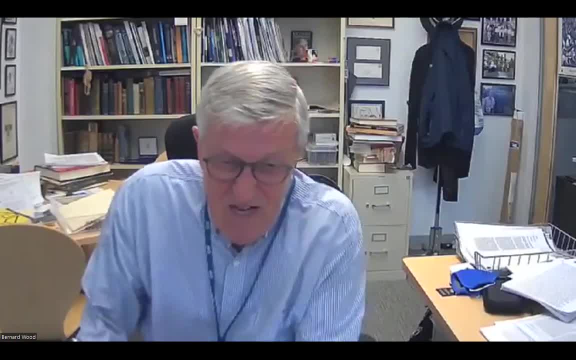 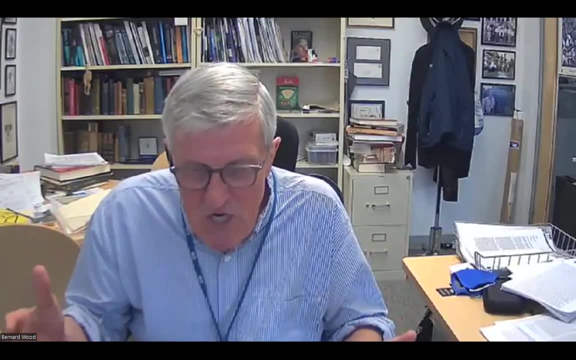 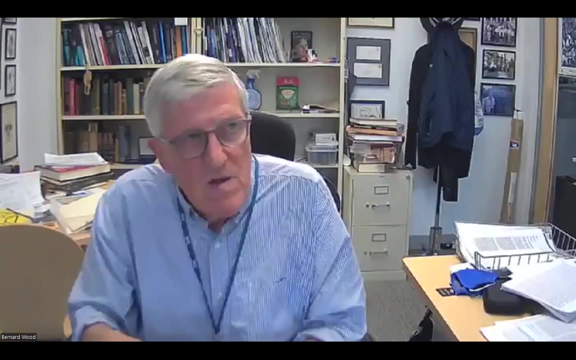 two species together than it is to split an inclusive species apart, and so it wouldn't take you five minutes to convert a speciose interpretation by saying, you know, by saying this is a junior synonym of this, and but it would take you much longer to take. 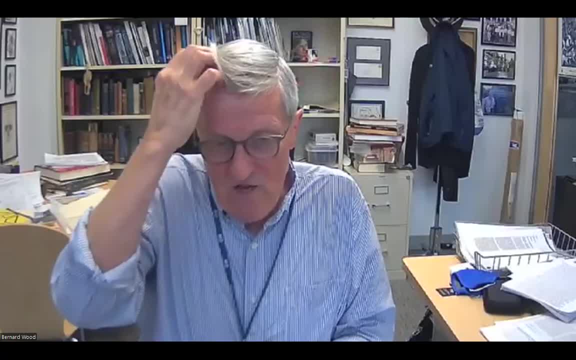 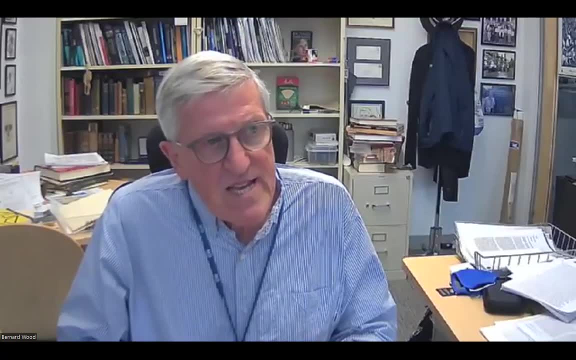 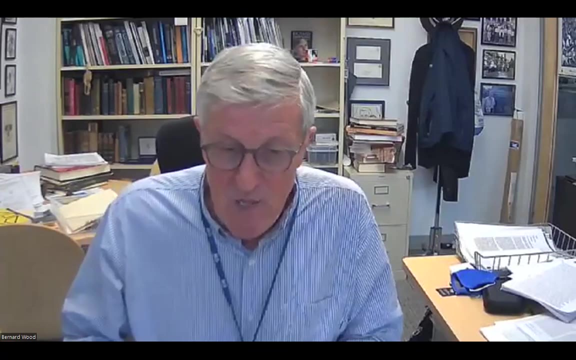 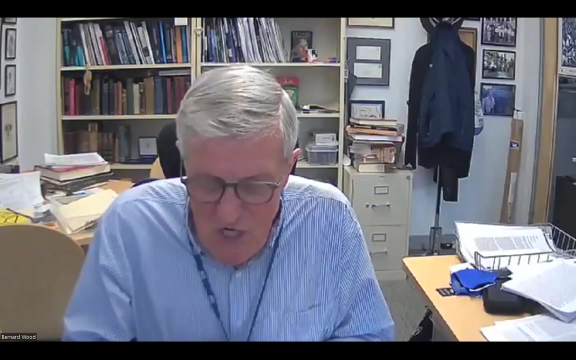 a lumping version and try and convert it into a more species interpretation. so one of my preferences for at least recognizing on a diagram a larger number of species is because it's much easier to lump them all together, you know, to lump them together and make pure, inclusive species, while continuing to follow the rules of the international code. 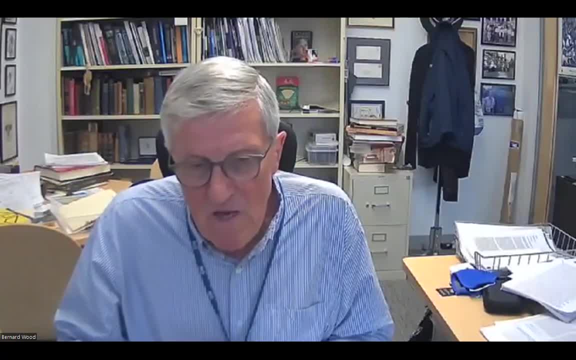 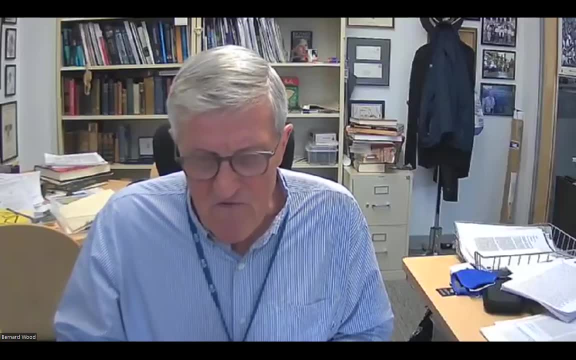 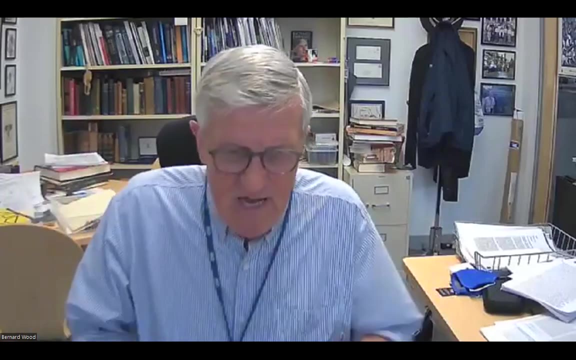 of zoological nomenclature, and as boring as those rules are, unless we have the right to do so. we have a set of rules we end up with. you know what we had recently? oh well, let's. you know, we don't understand homo heidelbergensis, so let's just give these things some new names. well, you. 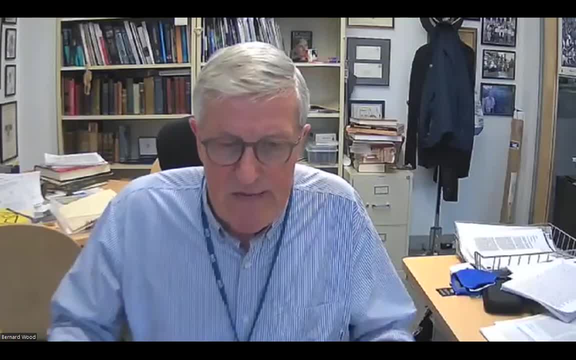 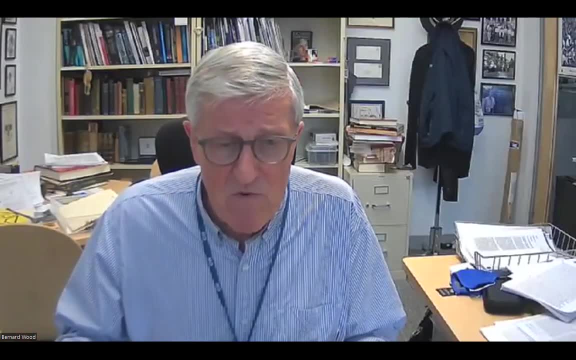 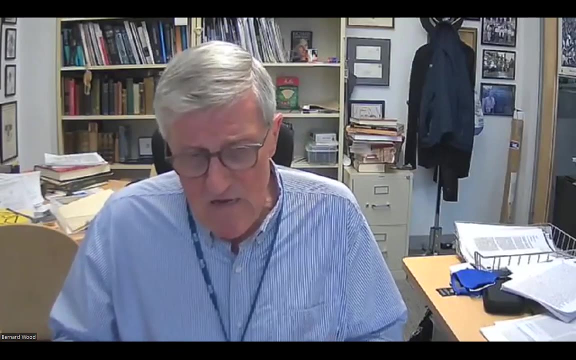 know, the problem with that is that, that, that that it flouts rules. and once you flout rules, then where do you stop? um, so that's my reason for thinking, you know, in sort of species terms. um, i really don't know. you know, i mean, it depends. 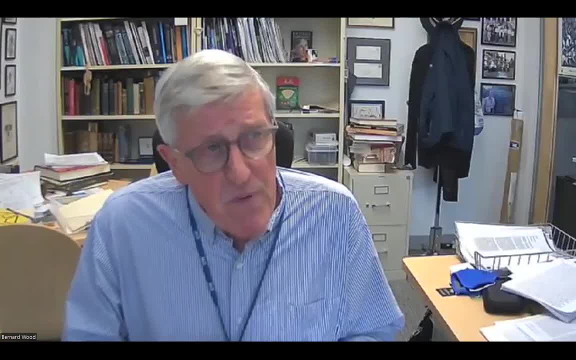 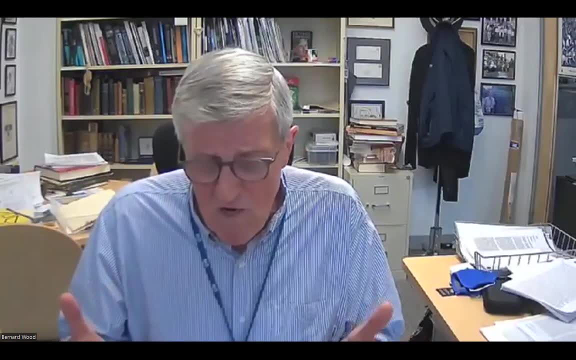 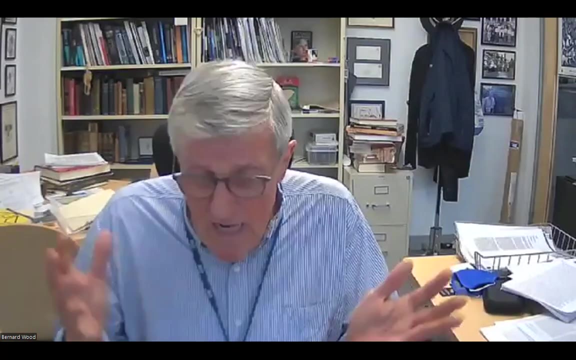 whether hominins were depends whether hominins were like carnivores, in other words they were pretty cosmopolitan, or whether hominins were were endemic to geographically restricted regions like lake basins or something like that. i don't know. i don't know, so i don't have a. you know, i don't have. 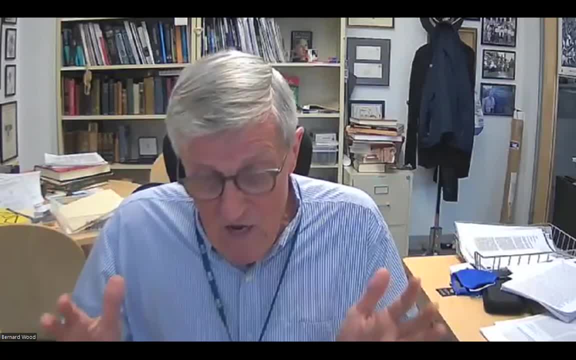 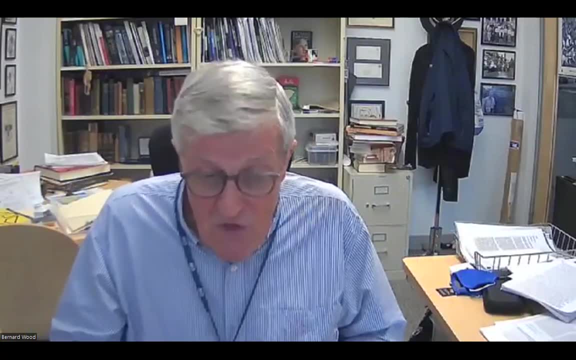 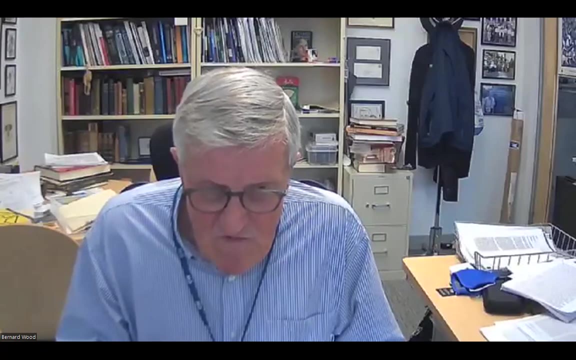 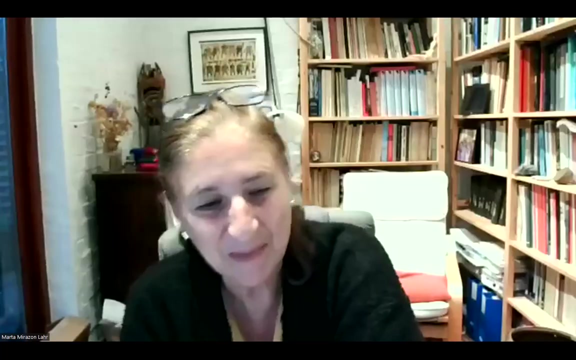 i mean, you'd have to talk to my therapist to work out why, why, why i'm inclined to favor a more species interpretation, but i just am for the reasons that i outlined, because it's much easier to to change it. thank you, bernard. i enjoyed the talk and i enjoyed the questions. can i follow up on dylan's? 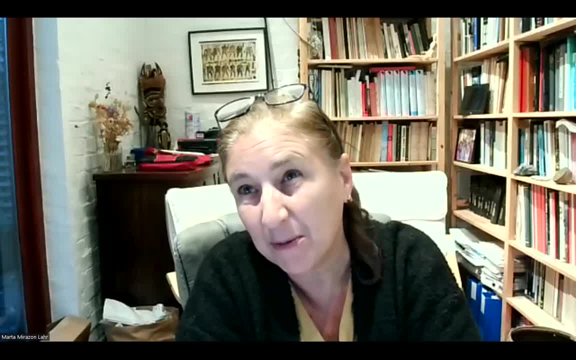 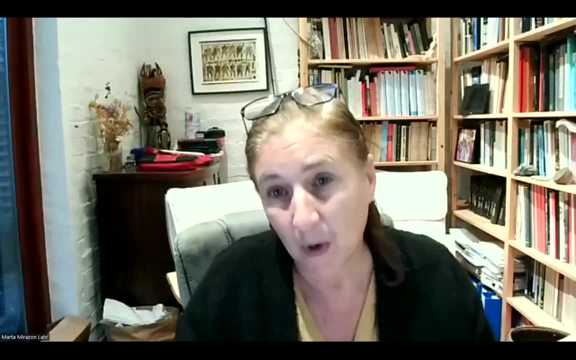 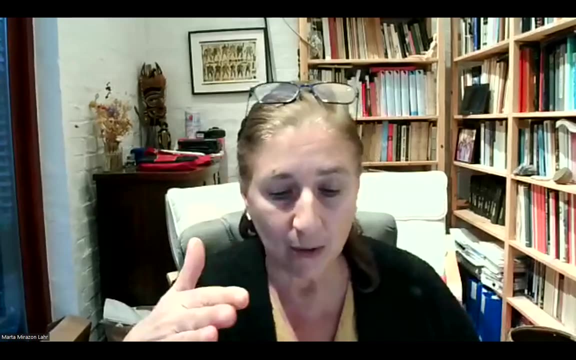 um, i agree entirely. i think that esp shows solutions, give us analytical power in a way that if you lump everything in one, you cannot get it. trying to untangle and understand and uh, but then what do you do? so, following your, your advice in the talk. so what do you do? 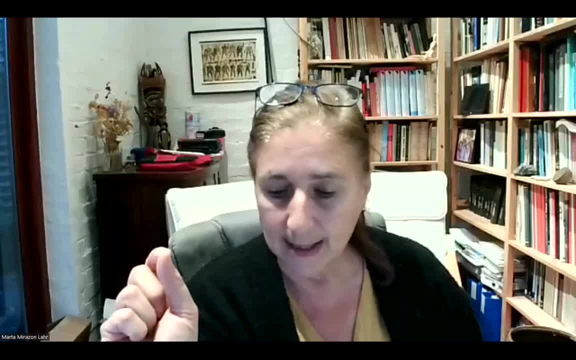 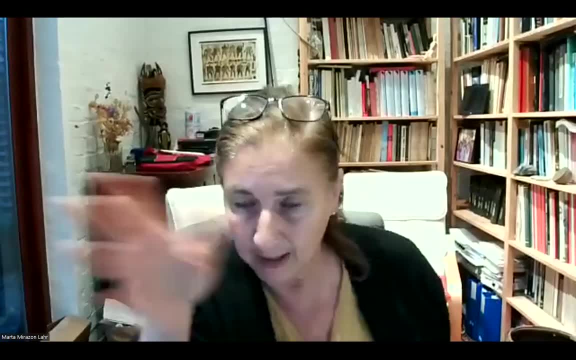 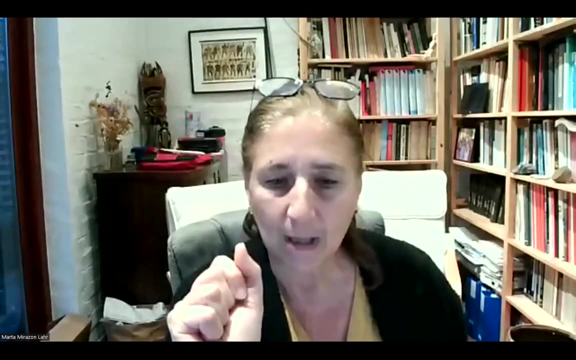 that people say: okay, so let's play with the idea that there's a unit called homo bodoense, for example, in the middle place, to say they don't like rhodesians of collie rhodesians and helmie and heidelbergensis, so where do you um stop with your narrative saying i don't? 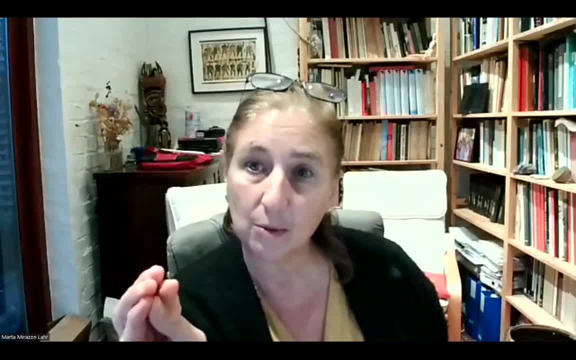 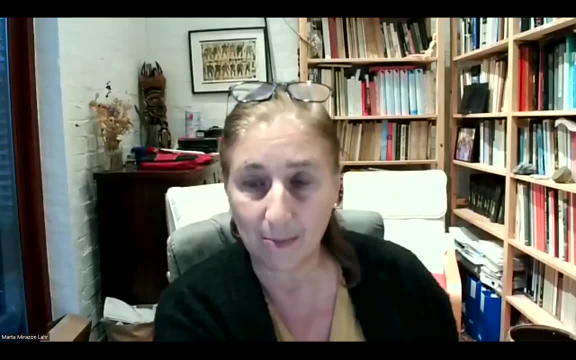 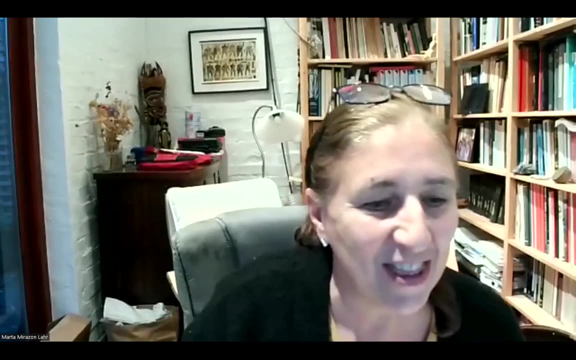 mean this to be a species, necessarily. i mean this to be a hypothetical taxon that allows me to explore if this diversity actually makes sense, if these patterns have correlates or not. so what would you do? would you not give it a species name? would you go like chris- chris, you're there, i can see chris there. would you go like? 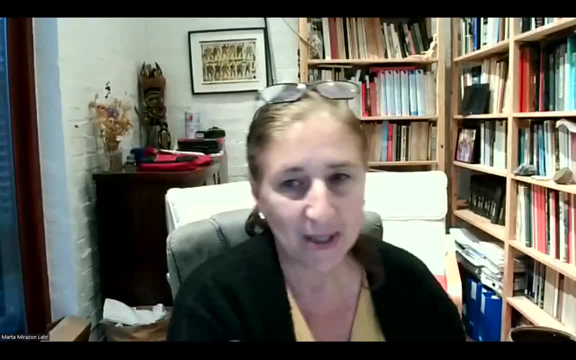 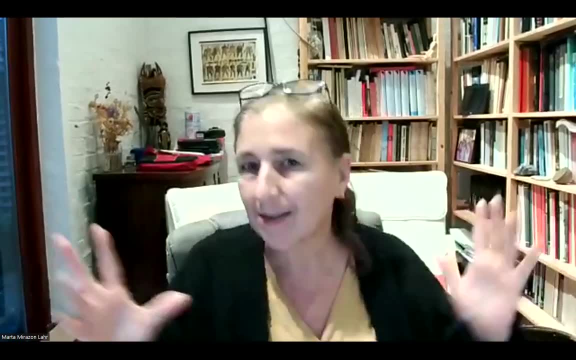 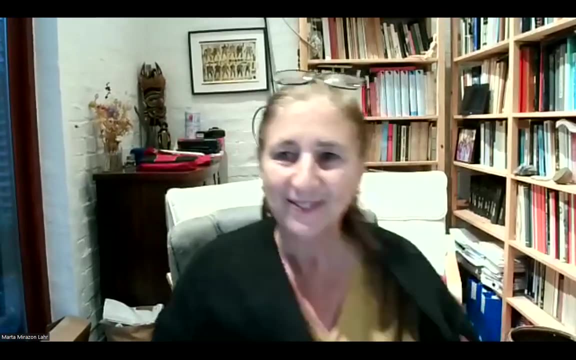 chris and say, oh, we have to talk about derived homo sapiens and uh, and and so on. so what do we do? do we qualify semantics in vernacular language or do we give it species names? and, chris, i'd like to hear you as well. okay, i mean, my sense is the following: you know, i am not a smart person. my sense is the following: we know species exist. we struggle to identify them when we have behavioral evidence, when we have morphological evidence, when we have genetic evidence. so we struggle to identify modern species even though we have orders of magnitude more information than we do about hominins two million years ago. 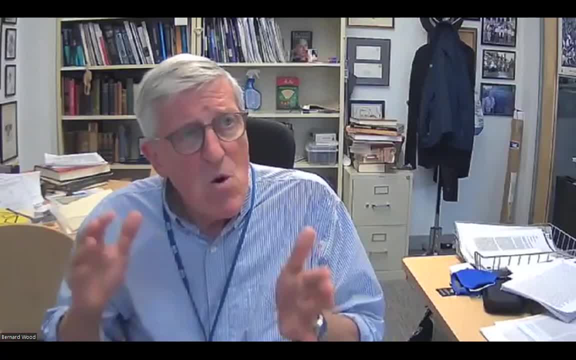 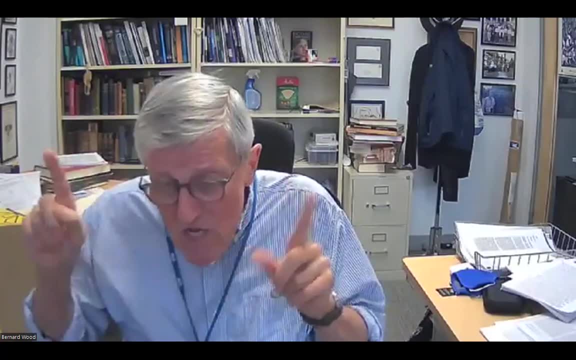 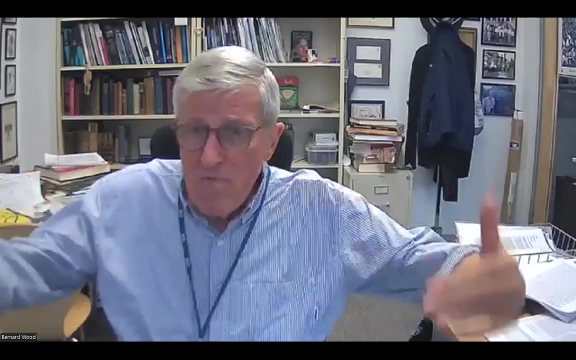 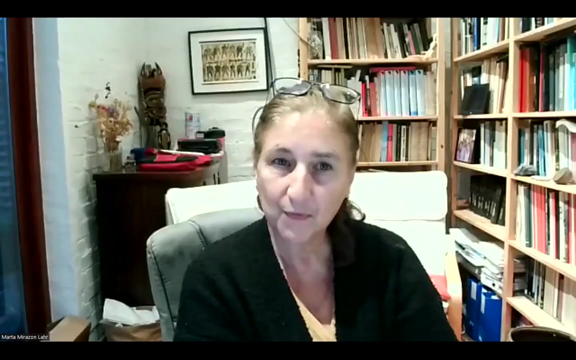 ago. so so we know species exist, we know they can be identified, we know that they are discrete in a sort of qualified sense, and so, therefore, two million years ago, we assumed that species existed as well, but they were discrete in the same way. and so you. my sense is that you can use. 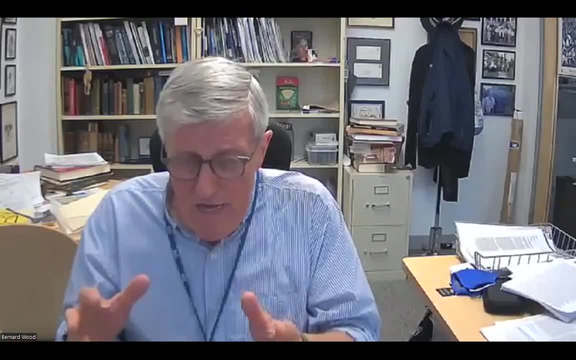 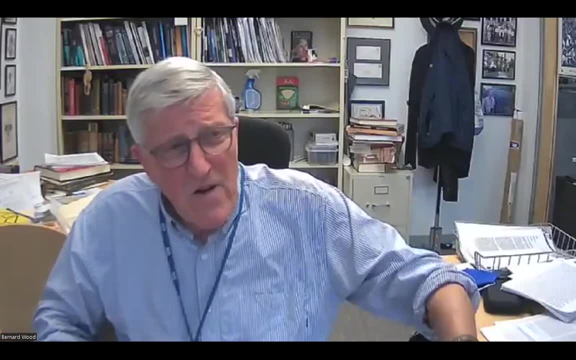 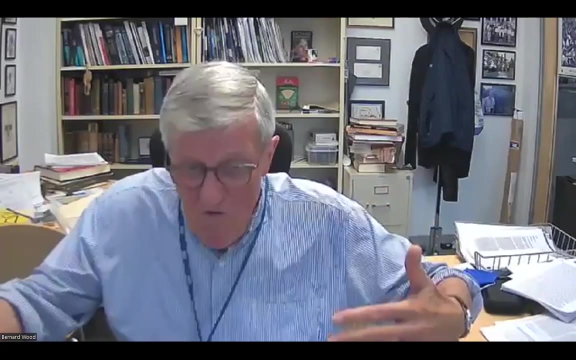 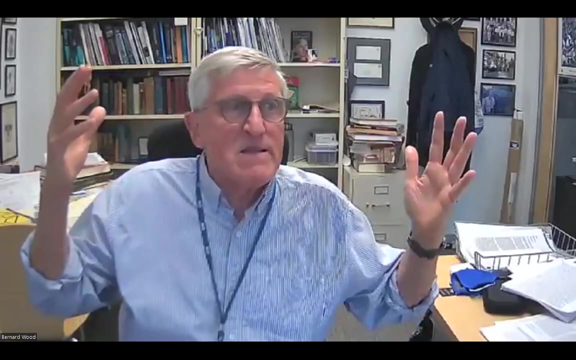 formal nomenclature to identify. i mean, you know, um, you'd have to be sort of crazy to think that oh7 was the same species as oh5, even though they had no morphology in common. yeah, yeah, absolutely, absolutely, absolutely. but you know, you just look at it and say: you know, will i ever live, if i live a million years, will i? 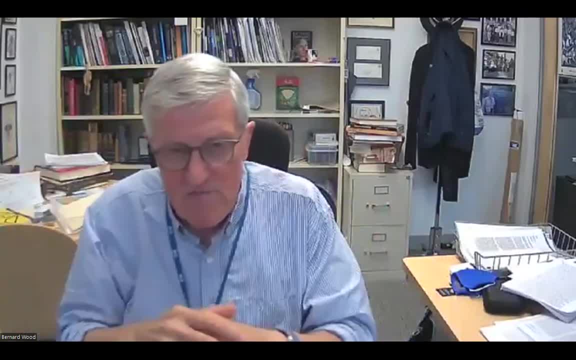 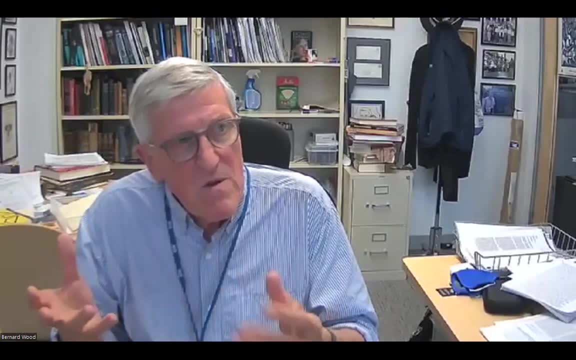 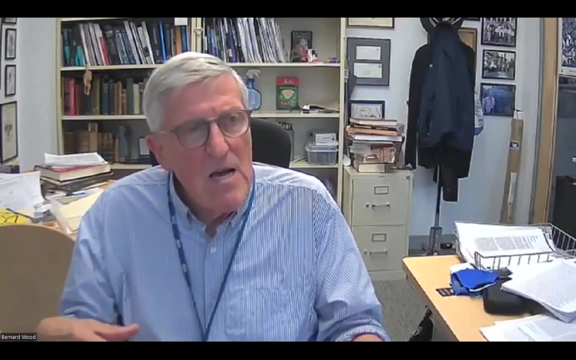 ever see a chimpanzee that has that cranium and that mandible? and the answer is no, yeah so. so there is a sort of you know, reducto ad absurdum, you know sort of sense to this, but my sense is that you know there's no harm in recognizing species, but you know, when you come to things like you know what's. 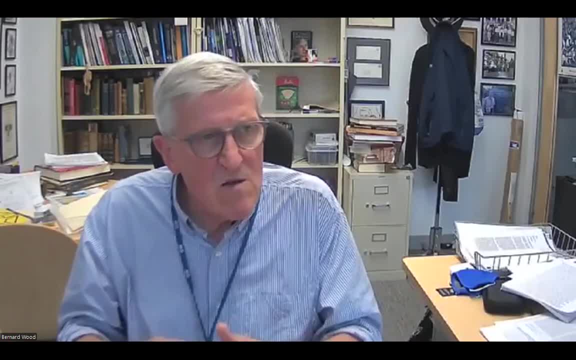 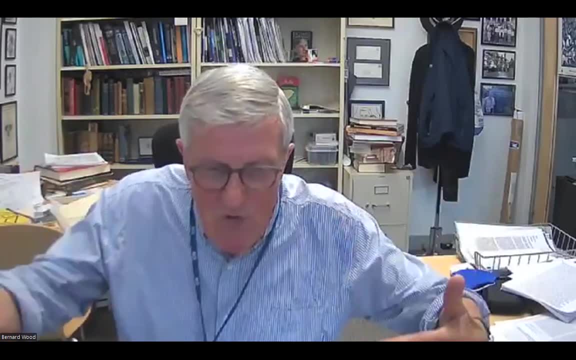 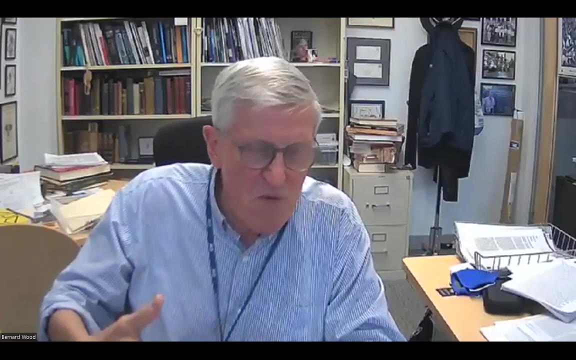 going on? what's going on at dimonisi? what's going on at the sema de las huesas? i, you know, i don't know, let's you know. for the time being, let's just sort of talk about them as as site samples and then, if somebody comes up with a positive argument, we can add those. 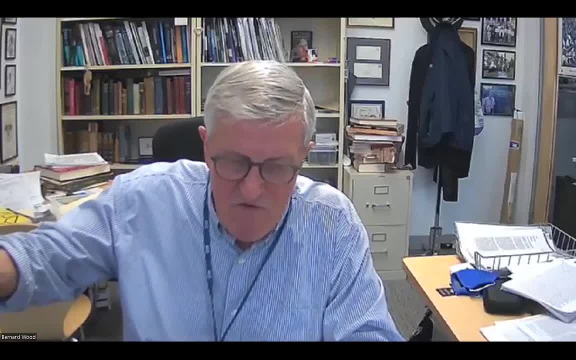 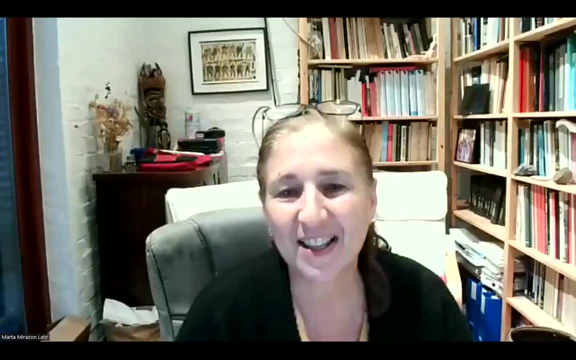 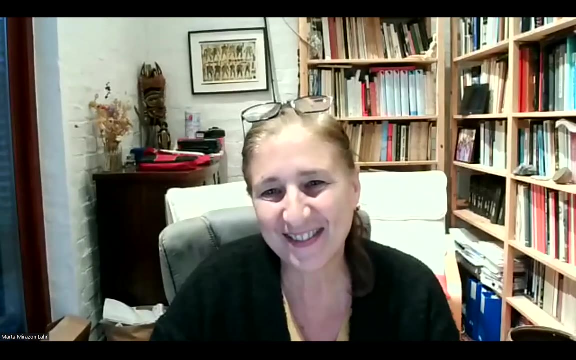 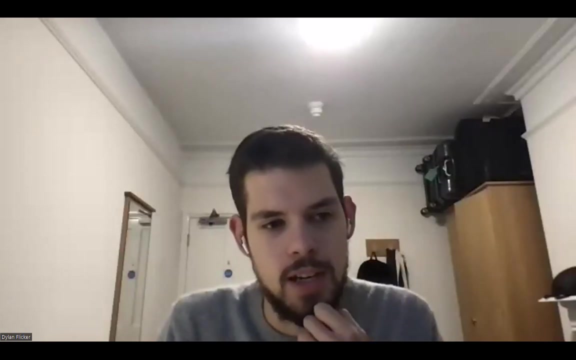 site samples to the hyperdimes, to the hyperdime of an existing taxon or we can recognize a new taxon. thank you, thank you. i can see that chris says that his microphone is not working, so he's listening only. yeah, i guess. i just have a follow-up to that which is there seems to be almost a reluctance. 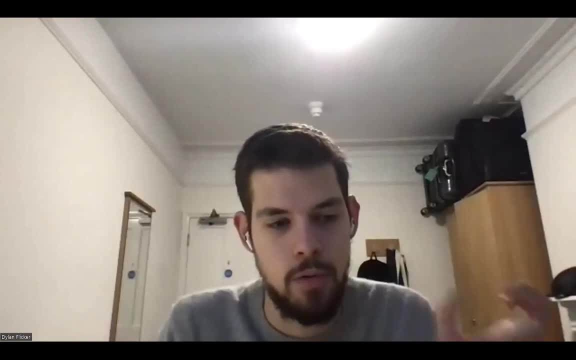 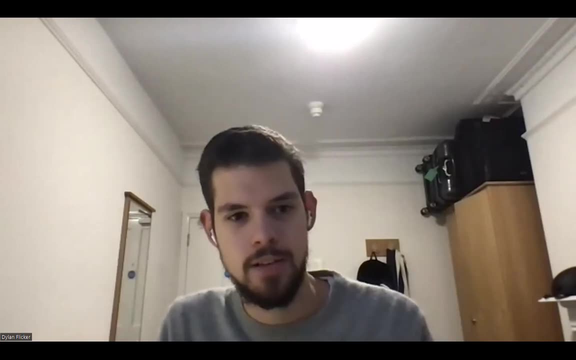 to use subspecies as a form of classification in the humming record, and i was wondering what your opinions on that are as like kind of a middle ground where we can address the degree of variation that we see, while also, you know, we can address the degree of variation that we see while also, we can address the degree of variation that we see while also. 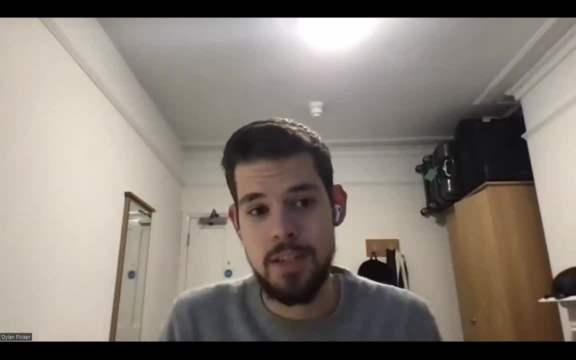 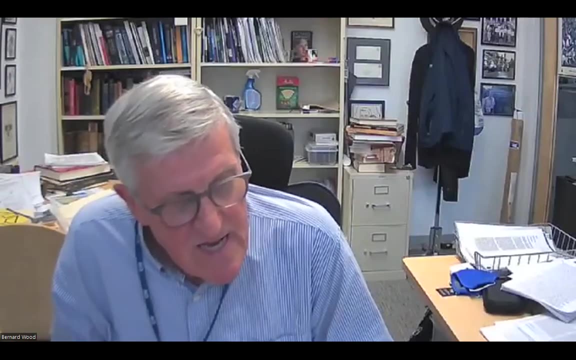 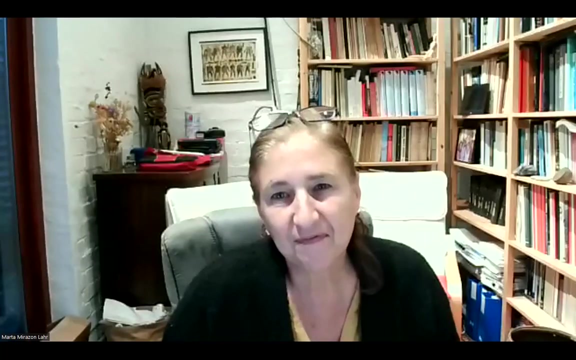 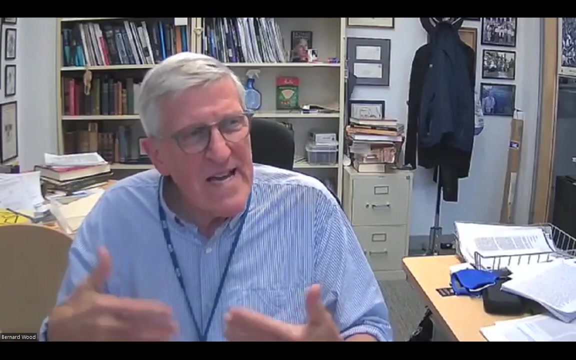 maintaining a degree of lumping. you are convincing me to be more of a splitter, by the way i'm. i mean, i think the problem with sort of subspecies is a is that it's an even more complicated problem recognizing species, and i don't want to give my uncertainty or my inability to you know to come to a conclusion. 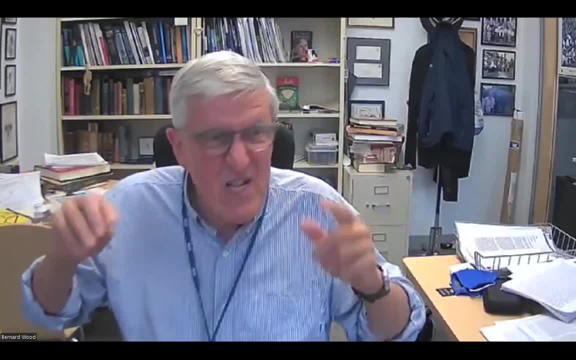 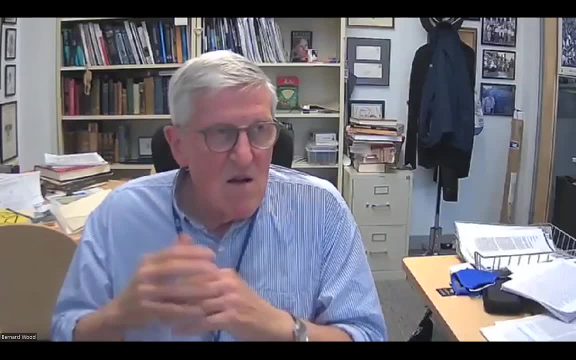 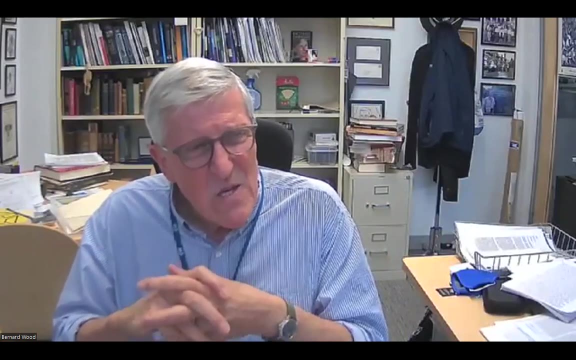 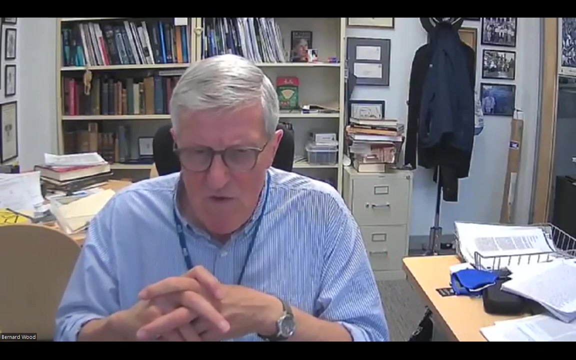 i don't want to make it sound as if it's more official and smarter than it actually is by giving it a, you know, a subspecific name. um, you know i'm not a zoologist and so you know my sense is that subspecies are used pretty sparingly, um, and i don't think we should adopt them as a sort of 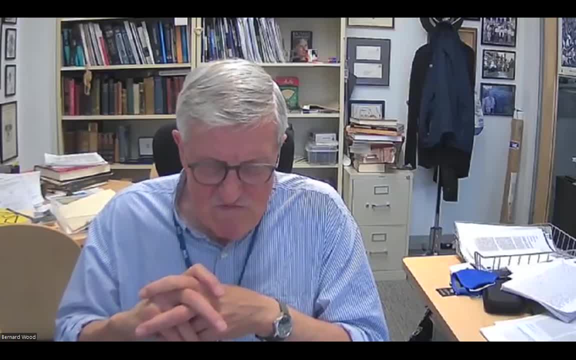 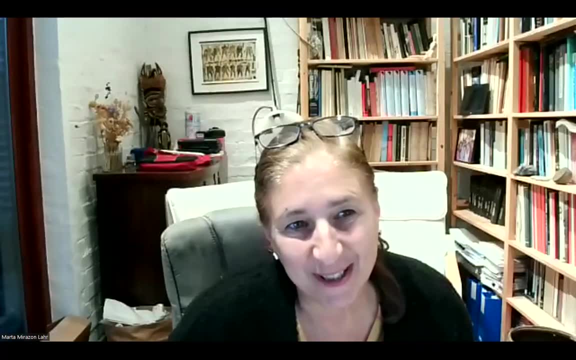 you know a cop-out, um, you know i'm not a zoologist, and so you know i'm not a zoologist and so you know i'm not a. i think that's such a valid point, dylan. so if you think that subspecies, which is a- 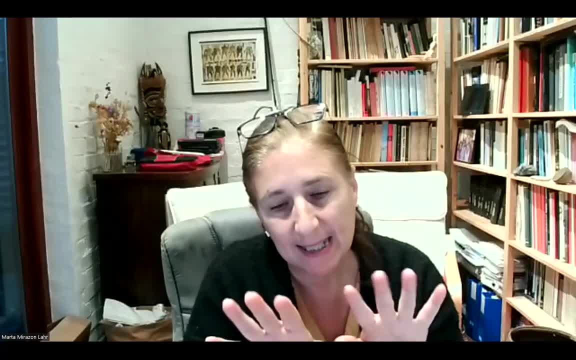 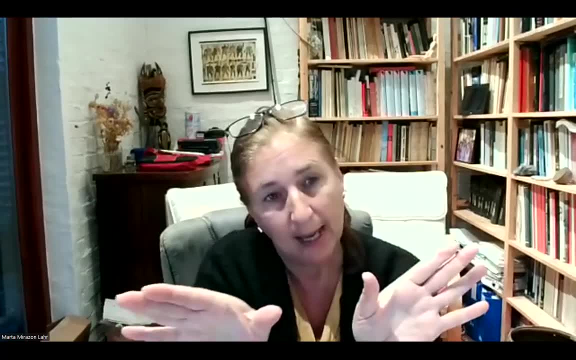 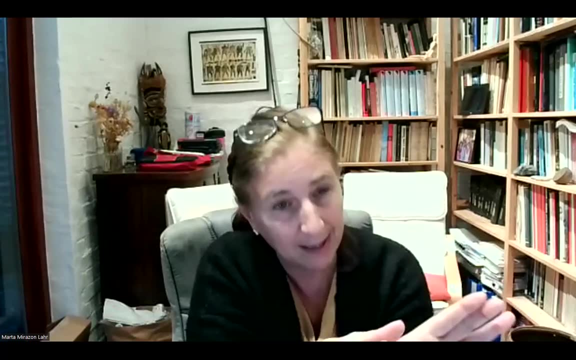 as a construct that we do to explain just shifting patterns of variation. it's overlapping variation, but with shifting levels of overlap. and you know, in paleontological species we just do not have a handle on that variation. that's population level variation, that's what subspecies is in the 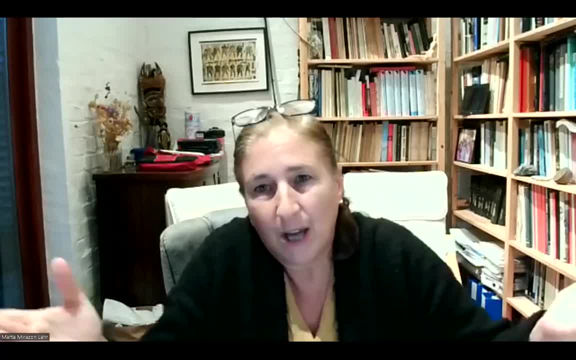 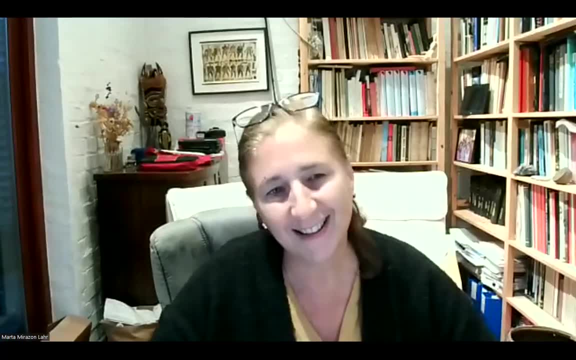 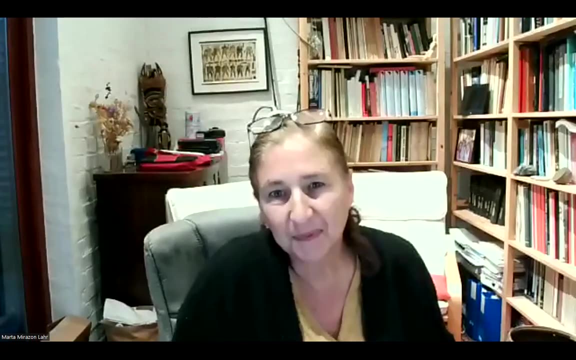 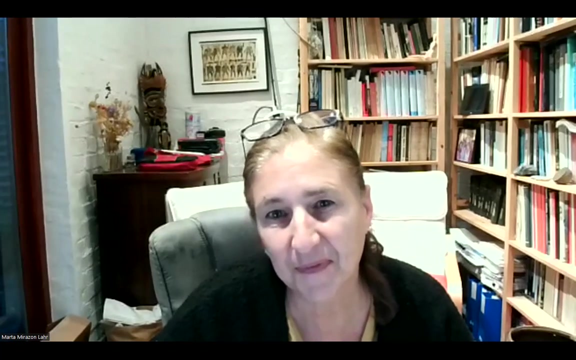 species is describing and i think we don't have populations to do it. so i think subspecies is a rush thing to do. and do we have any more questions from from any of the guests? uh, you're also open to send them to dylan or i and we'll read them out as well, but we've got a good discussion going. 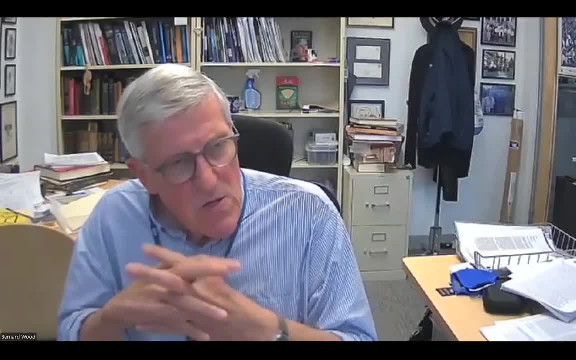 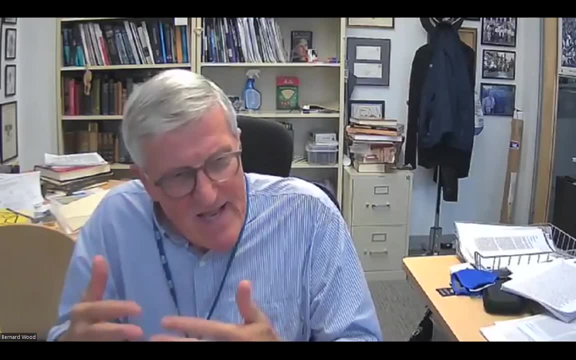 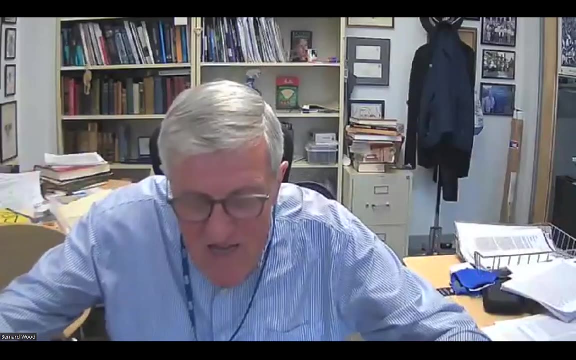 well, i'm sorry to be such an eeyore as as rob suggests. um, it's not that i mean to be an eeyore, but it's like an actor on the stage. unless you go on the stage and exaggerate, the people are not going to hear you. okay, if you just sort of go on the stage and 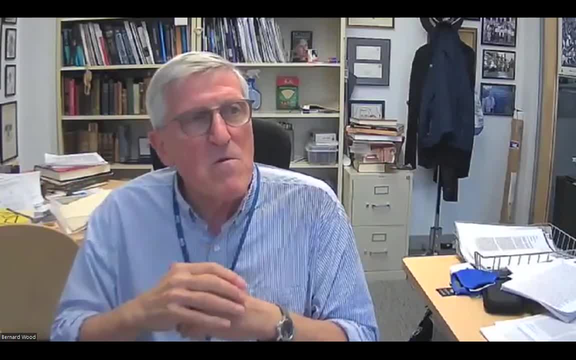 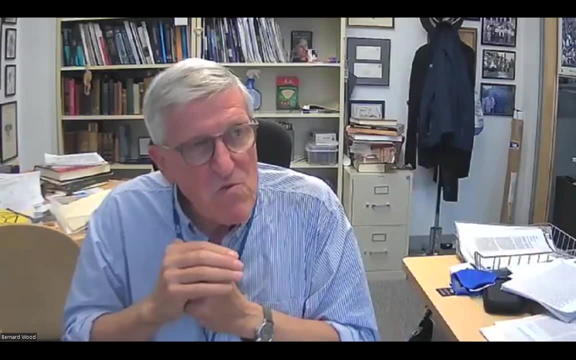 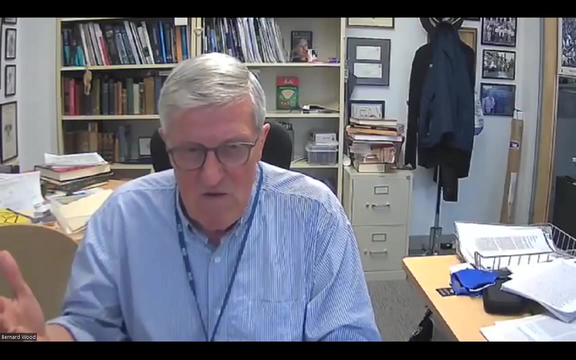 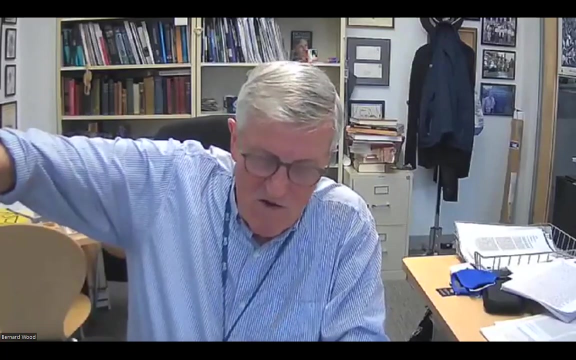 talk as you would sort of talk to a neighbor. so so, in order to make my point, i'm clearly exaggerating, but i want to exaggerate, but but the reason i'm exaggerating is that i want you to think about this, and you can think about it and then say: you know he, or go away, he come in um, and that's fine. 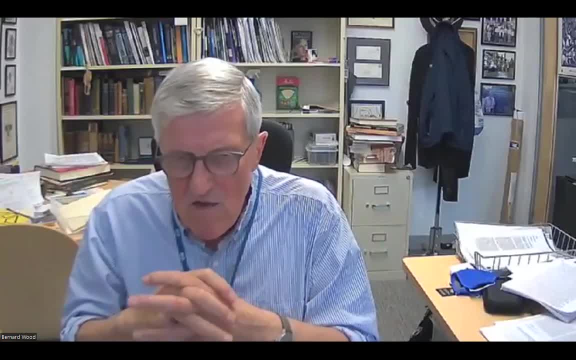 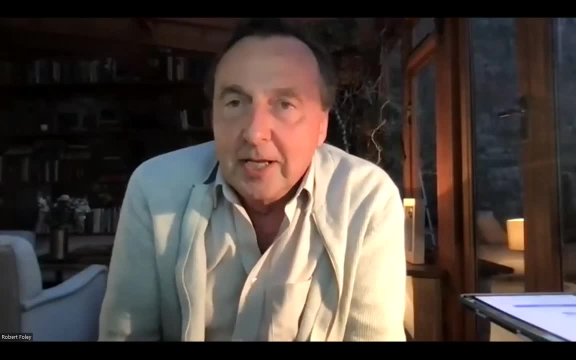 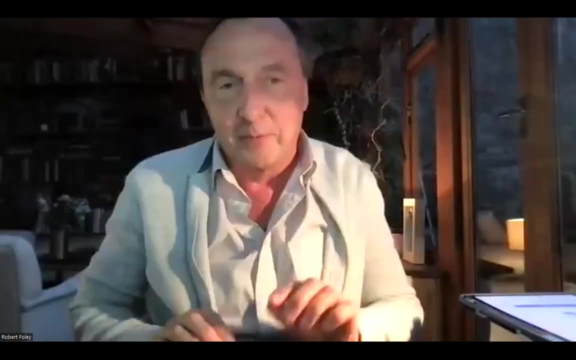 but i don't want you to make that decision without actually thinking about what it means. uh, let me just add, bernard, that of course, what winnie the pooh? you need both eeyore and tigger. i mean, the book doesn't. the books don't work without, doesn't work with one or the other. yeah, 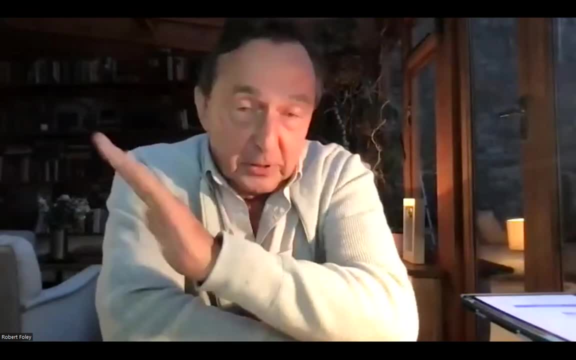 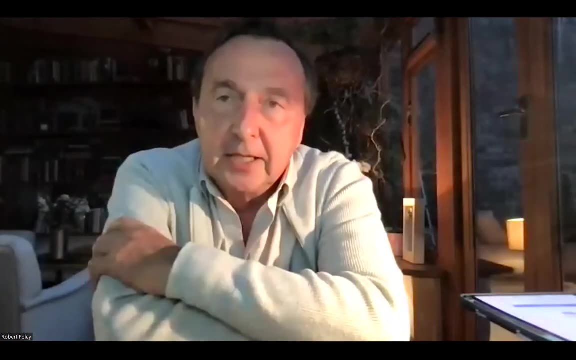 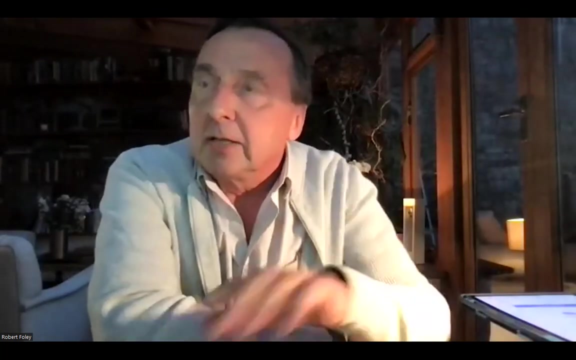 i know. but, uh, you know, i, i think, i mean, let me say i fully agree with you about the spesio's nature of, of the hominin record and and it's obviously, um, you know, clear, um, uh, it's what, it's the pattern we see and it's the pattern i think we would expect. i have a slightly methodological question. 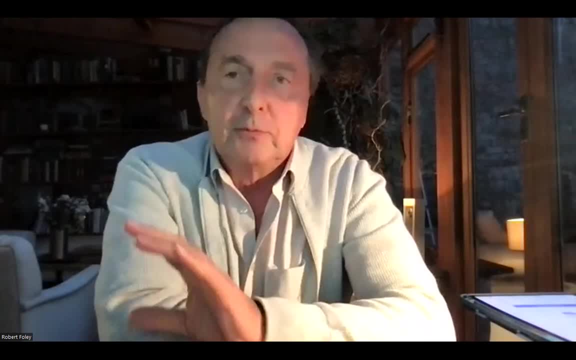 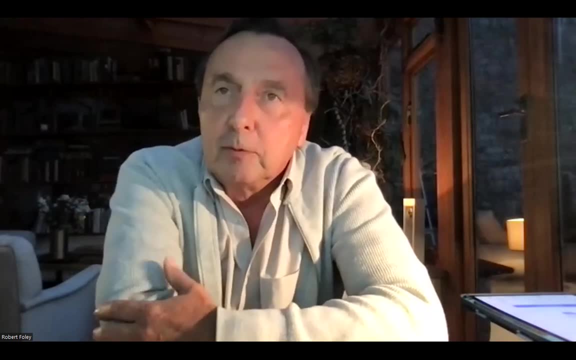 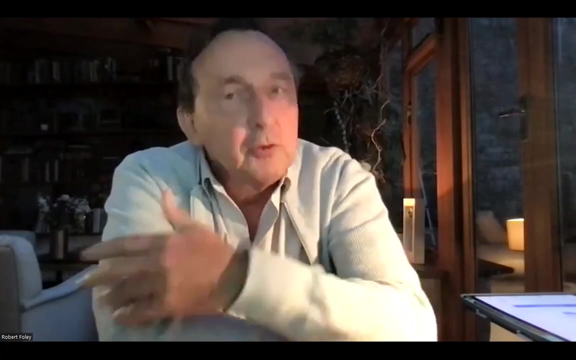 so i, i, you're, you're obviously arguing strongly for caution and i think that's absolutely right and there's, you know, a lot of exaggeration, but there's also a place for, you know, we could be a bit popperian and say: you know what about the bold hypotheses which then take us into new territory. 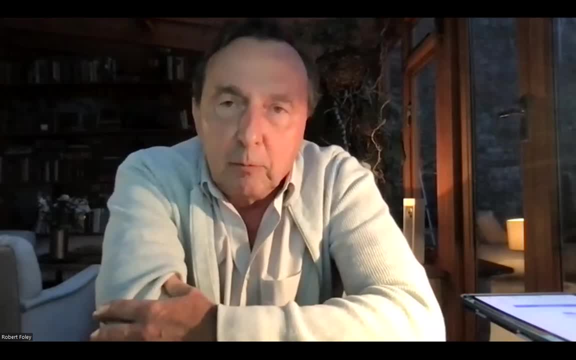 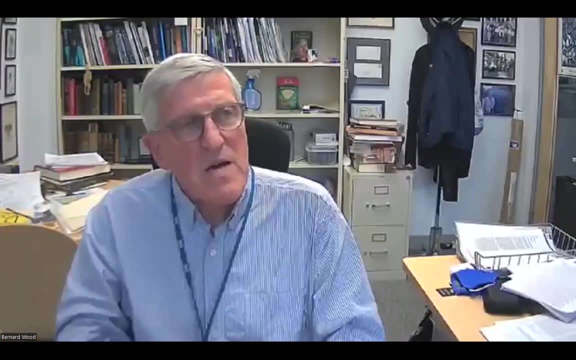 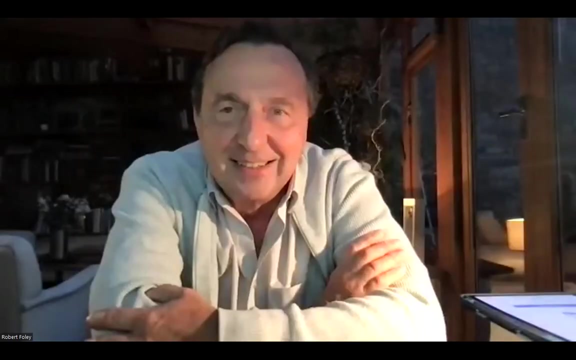 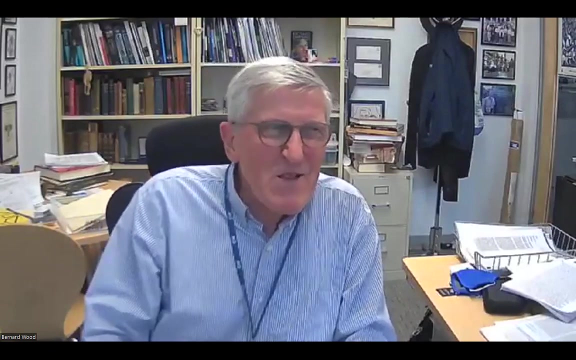 driving, driving the subject along and and, in a way, without those bold hypotheses, we might end up being a little bit stuck. yes, i mean, you know i'm that's right. i know that there was a hand raised by mark somebody to see. um, yeah, i mean i'm not against sort of bold hypotheses, but you must understand that i was educated. 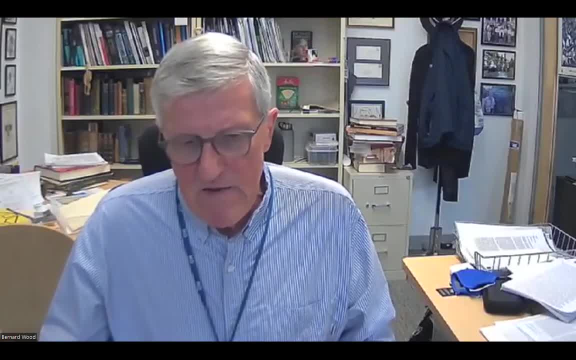 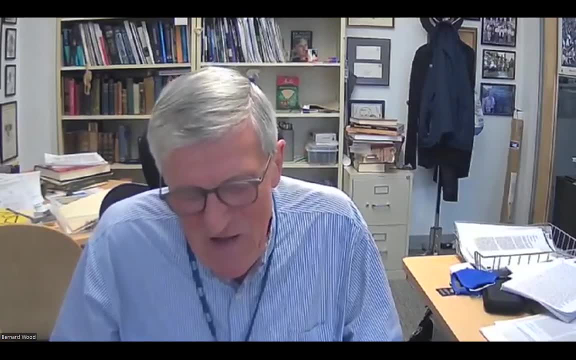 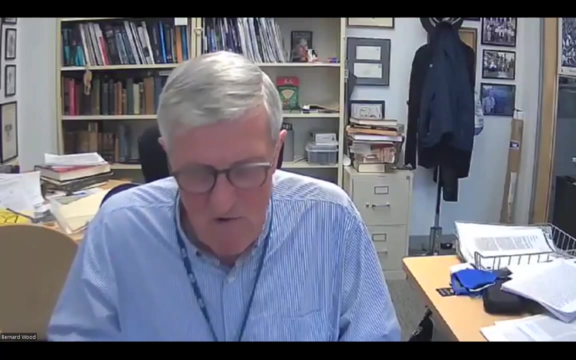 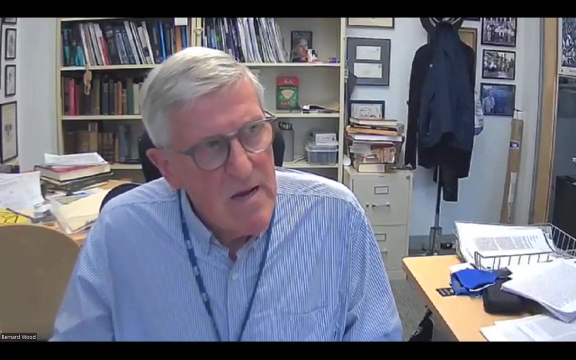 as a doctor, okay, and you know if you're in a hospital, nobody was interested in your bold hypothesis. uh, absolutely no one was a bold surgeon they were interested in. you know whether you had evidence, uh, you know, and so on, you know, and so i agree that the bold hypotheses are part of the weft and 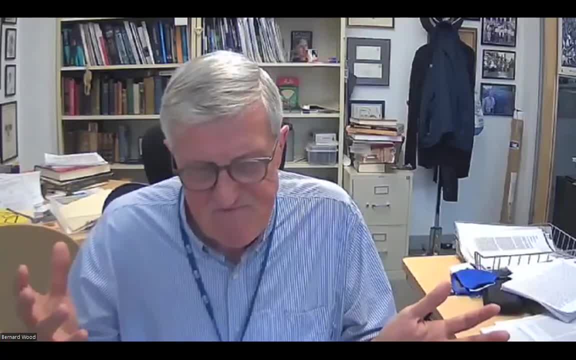 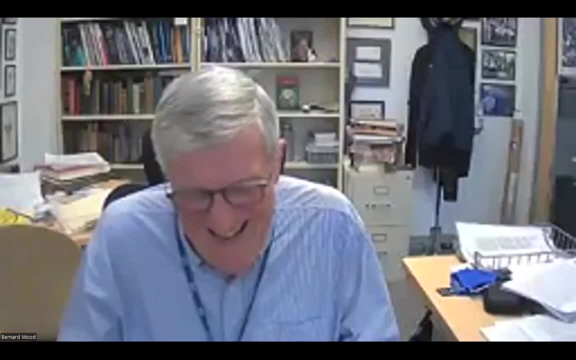 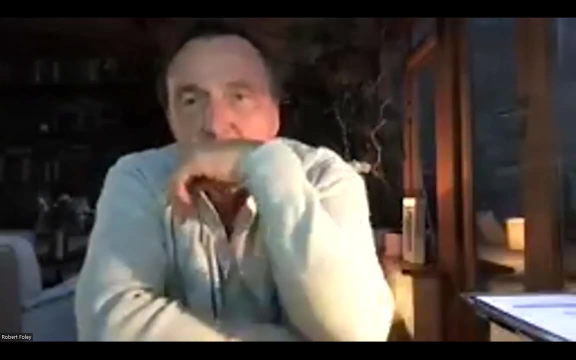 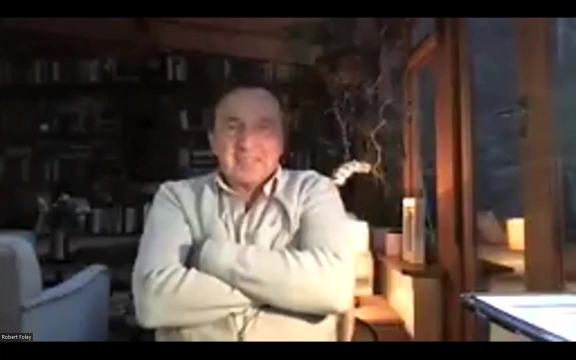 warp of what we do, but i think they're only part mark. good morning or afternoon or whatever it is. wherever you are, good morning everyone. hi mark um, hello everybody, um um. i wanted to try and push you a bit on this avoiding why questions, and you were pretty explicit there about trying to discourage people from 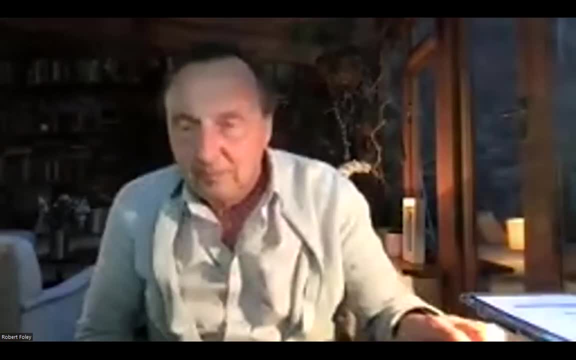 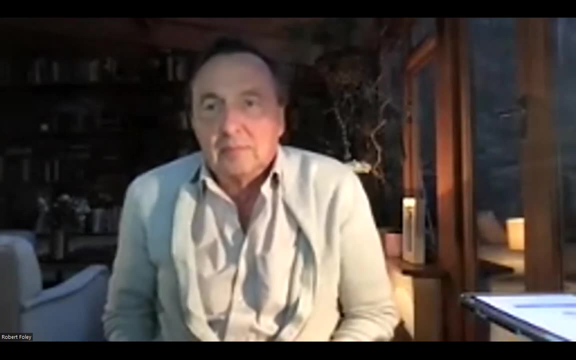 thinking about why questions? because they're they're difficult to to answer and i and i sort of understand the appeal of that position but i'm not sure is actually empirically valid. i mean, is it actually the case that why questions have proven to be more difficult in paleoanth than how questions? so if you look at for 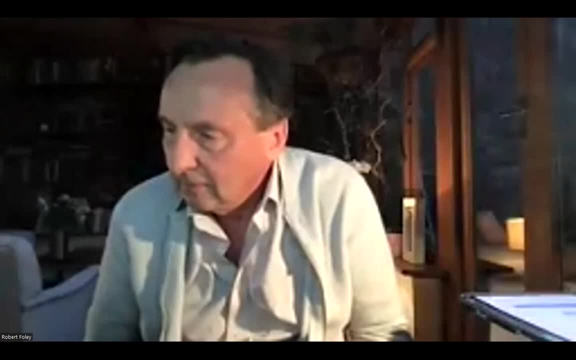 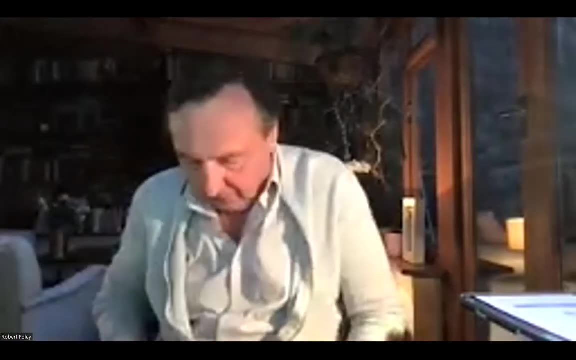 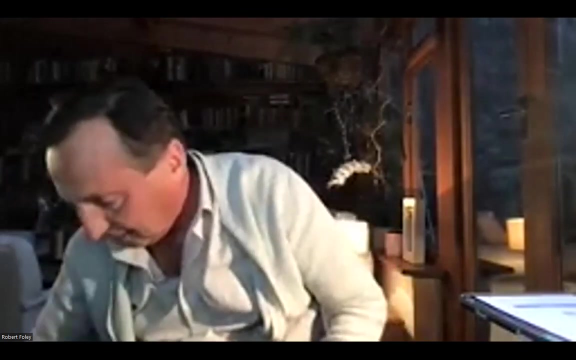 example, the uh, the debate, long-standing debate about how the australopithecines moved around, which is a how question. is it any more resolved than the why question of why bipedalism arose? i mean, i don't necessarily think there's an obvious difference between those two questions. 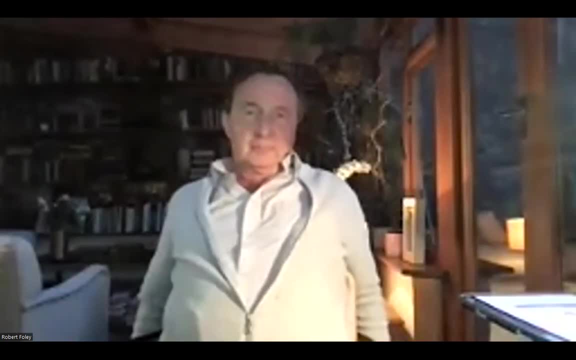 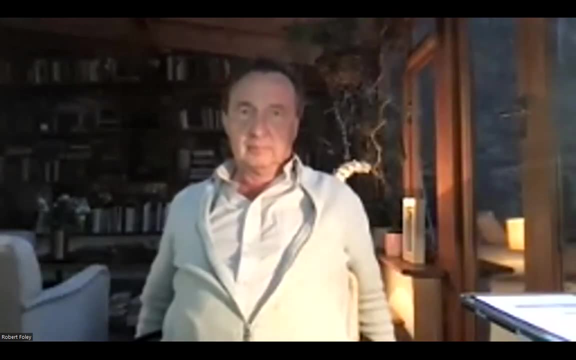 in terms of their how, their degree of resolution or the degree of consensus about them. and on top of that, i think the why questions actually quite often have driven research in a very productive way. that how questions, uh, you know, quite often don't so, for example, thinking about, uh, climate change as a driver of of human evolution, that that's. 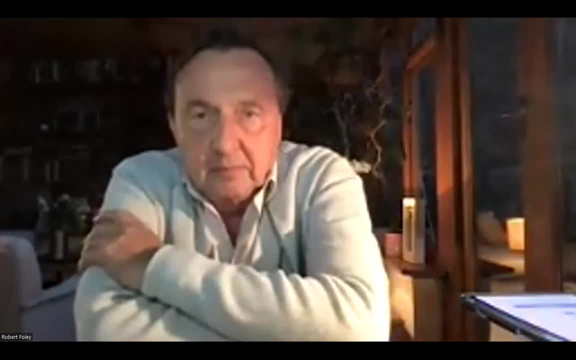 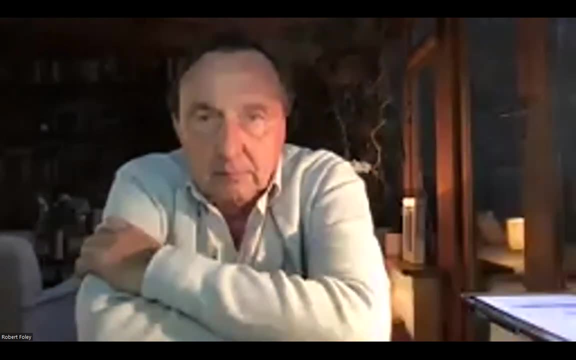 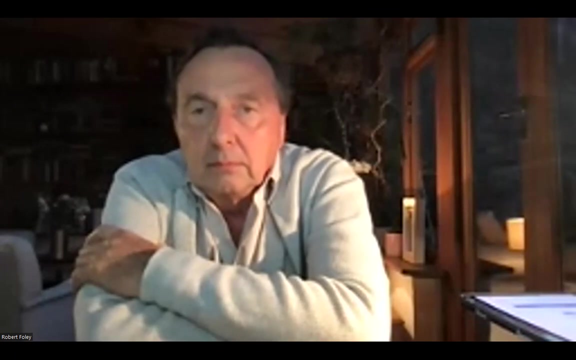 and obviously uh resulted in a huge amount of research and it's a why question and it's been very productive to to think about the potential drivers of human, human evolution. you know, the why questions are, i think, actually uh worth investing time in, so i would just want to you know, see whether i can provoke you to say a bit more about that. 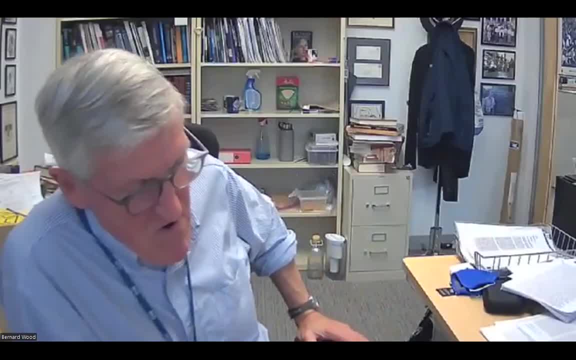 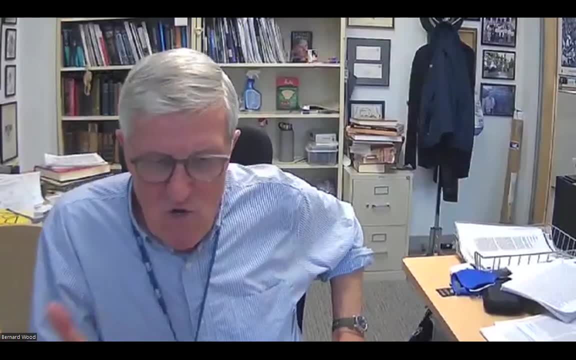 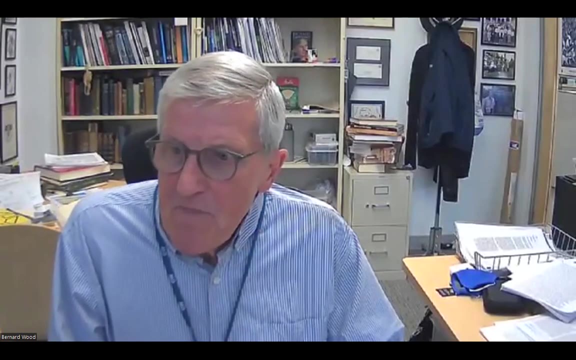 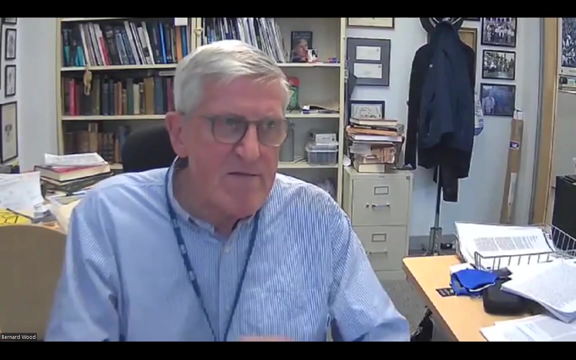 well, you can provoke me. it's nice. it's nice to hear you the, the, the my my sort of caution about why questions is largely directed at graduate students, because i think, um, you know, basing your thesis on a why question is is a bit like you know. 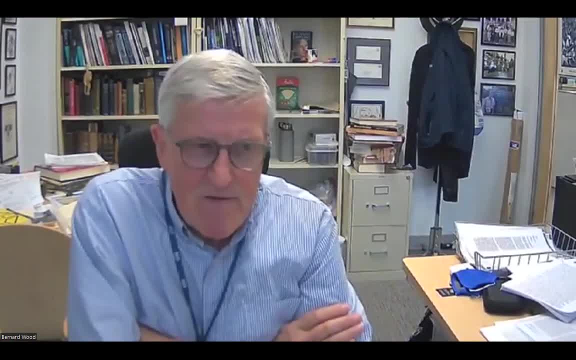 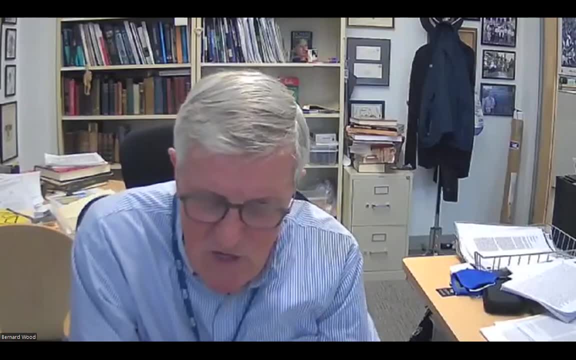 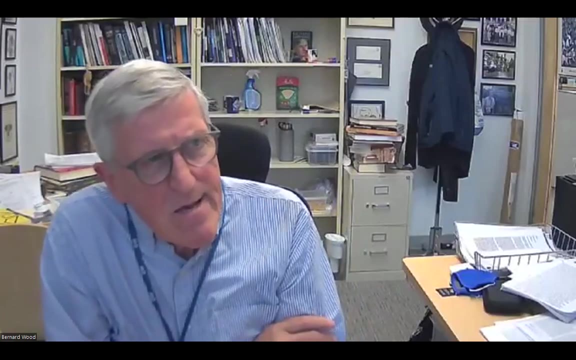 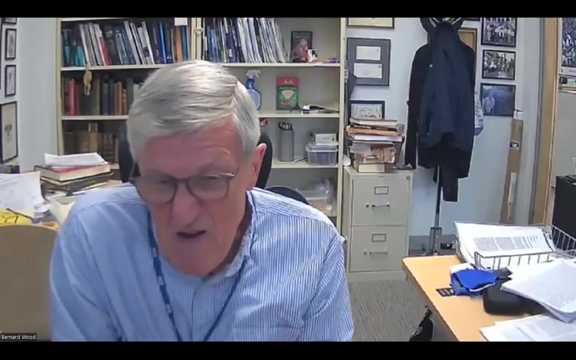 beginning to learn to be a circus acrobat by going straight into the you know, the most you know, into the highest um part of the tent and that sort of thing. my sense is that why questions can be asked. i think you know, for example, why questions are a. 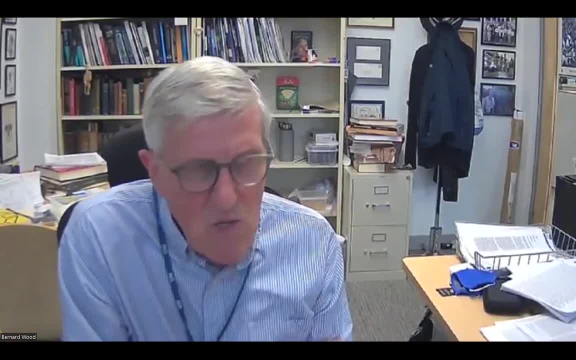 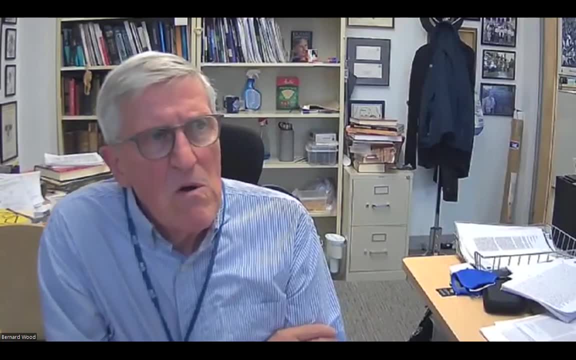 good way of generating research support. because i think that's a good way of generating research support. because i think that's a good way of generating research support, because i think that's a good way of generating research support because, um, because organizations like the nsf or research councils in the uk or in canada, 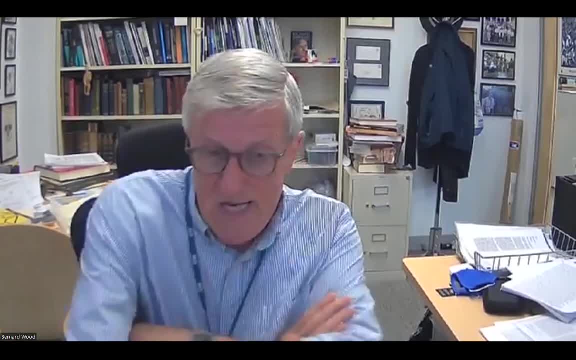 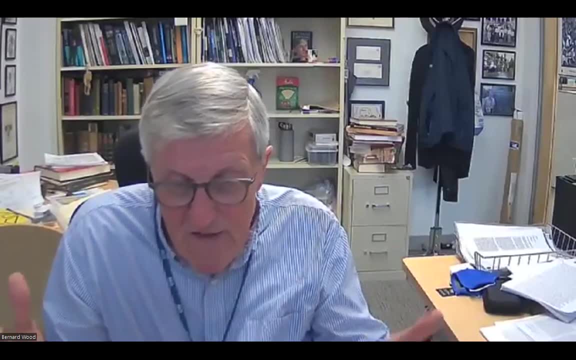 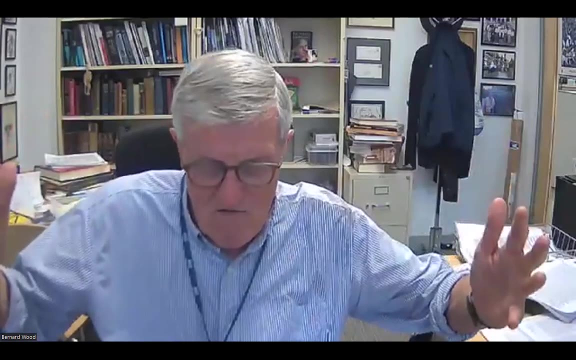 they, you know they like the why questions because it's, you know, it's, it's, it's, it's, um, it's. it gives them something to tell the politicians: oh, we're trying to find out why, okay, and the politicians can understand the word why. questions are a good way of generating research support because 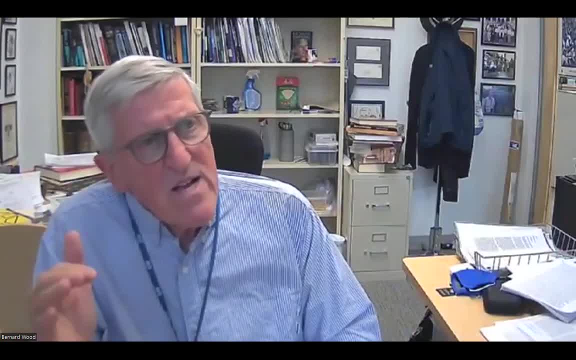 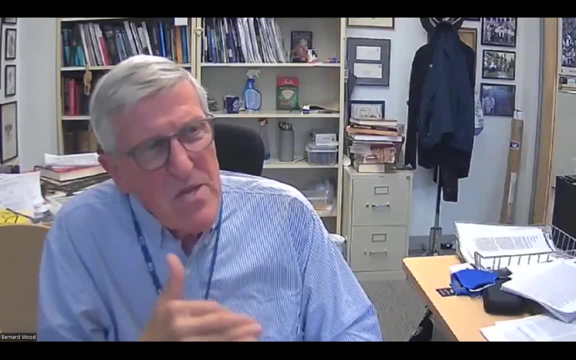 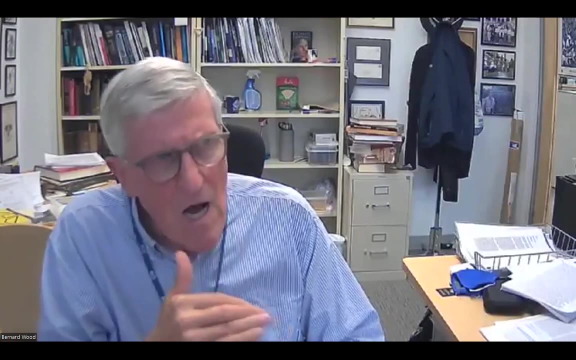 we're trying to find out why. okay, and the politicians can understand the word why. so i've got nothing against why questions? but i but as a personal but, but it's questions to drive somebody's personal research agenda, then i think it's, it's a bit risky, um, and i think to say that 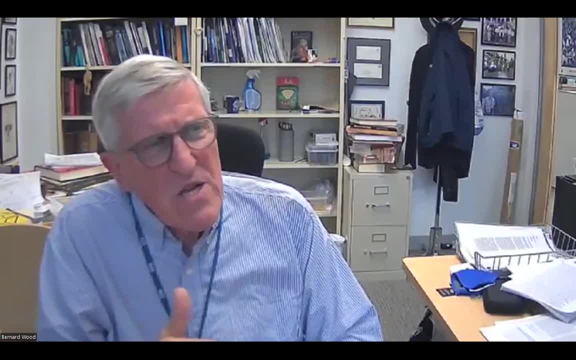 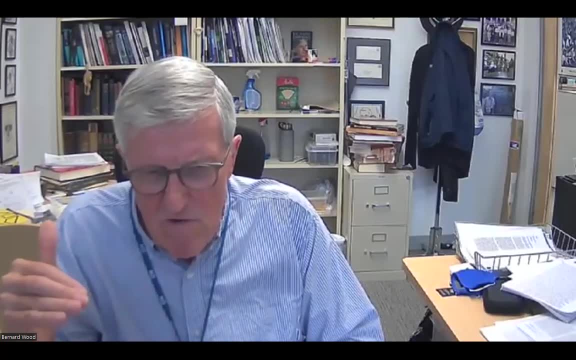 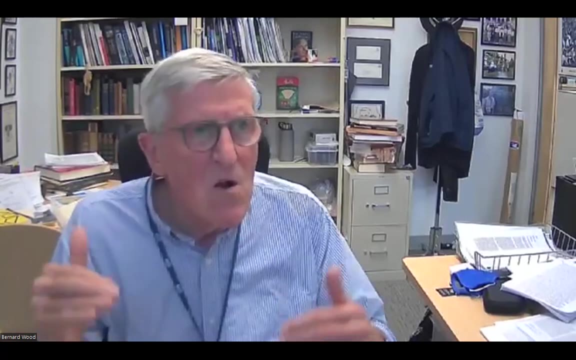 well, you know how questions are often as risky as why questions is is not a reason to well, you know how questions are often as risky as why questions is is not a reason to give people license to answer. to ask why questions and libertum, why questions are very interesting. 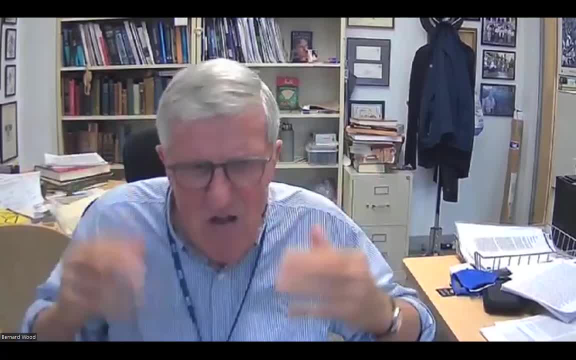 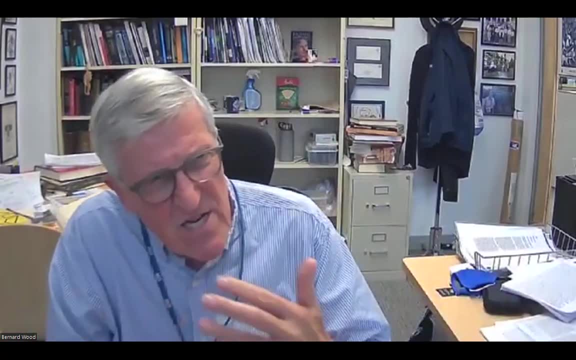 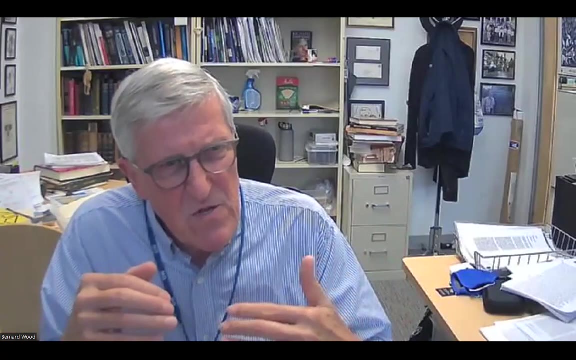 you know, of course, you know, i would sort of desperately like to know why did peranthropus become extinct, why did this and that sort of happen? but when i actually try and convert those informal questions into a scientific um, into a scientific program, then i think that's. 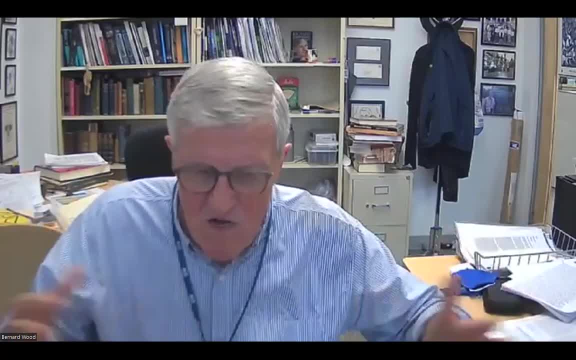 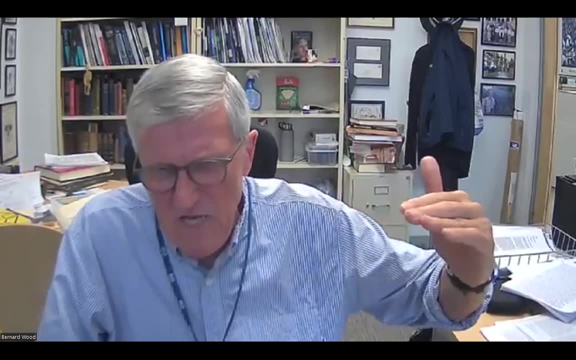 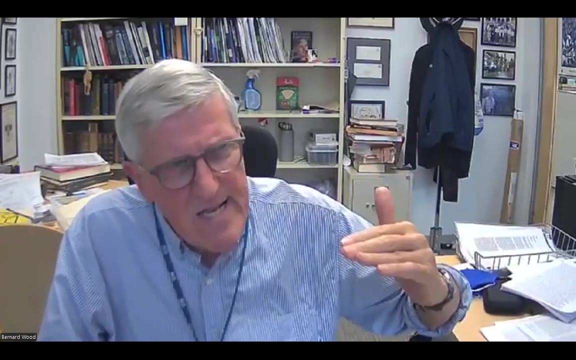 i think that's the best i can do. so i i think that that's the case, but, but i think i'd like to think that's the case, but, but i have difficulty doing that. i have to go back to how and to and to come up with, say: okay, you know there are maybe four, eight for competing explanations. how can we? 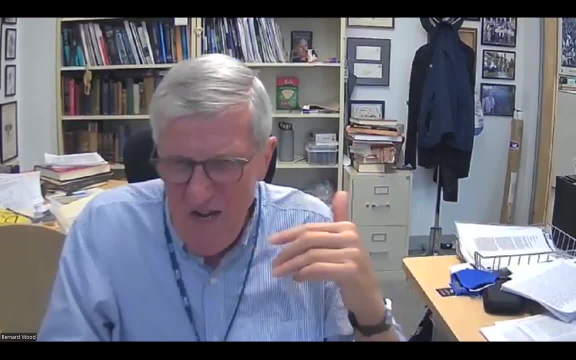 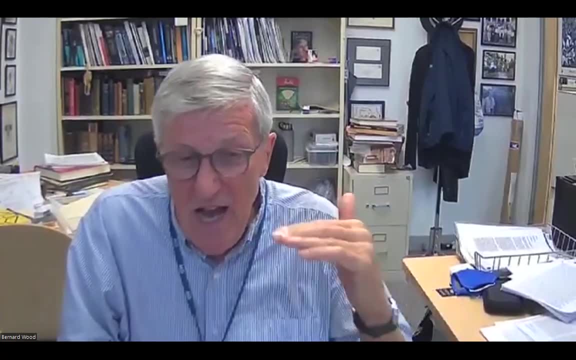 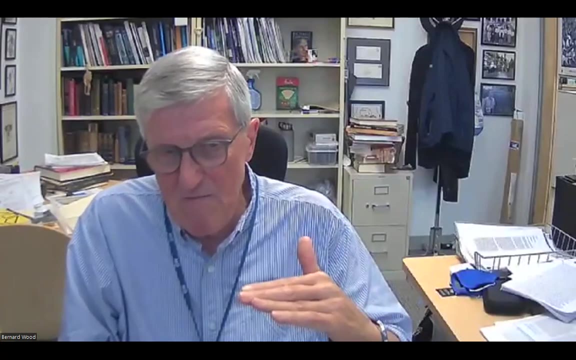 try and eliminate the least likely. and my sense is that what i've been trying to do about human evolution is not to find out what happened during human evolution, but just to reduce and to try and eliminate the less likely things. But I don't think I'm going to alight on what happened. 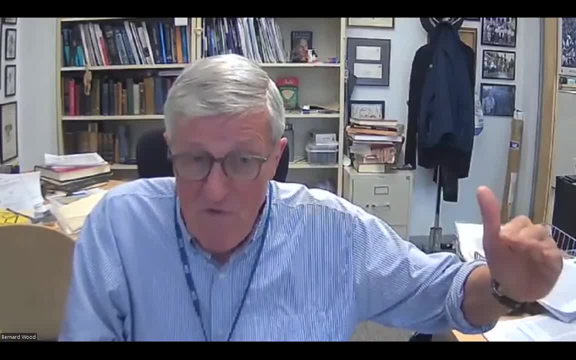 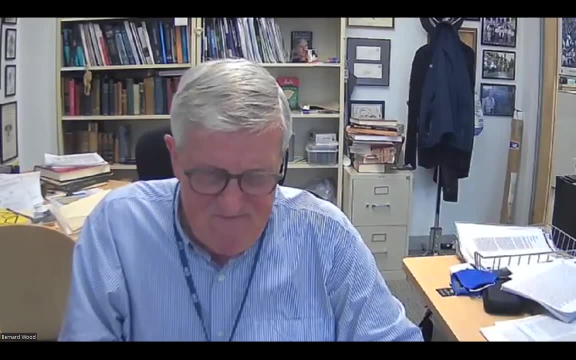 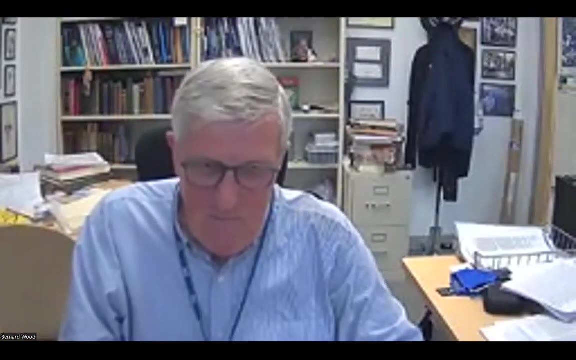 but I'm going to get closer to a short list of things that might have happened. Not sure that that's going to satisfy Mark. That was a good answer, thank you, And if we have no more questions, thank you, Professor Wood.